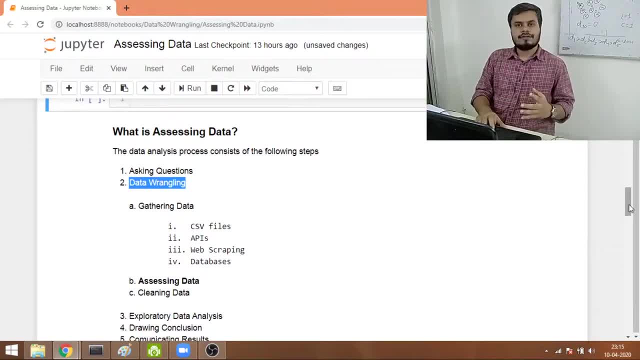 so, guys, we are in the process of learning data analysis process and you already know there are five steps in the data analysis process. the first step is asking the right question, and you already know that did. this varies with individual. this varies individual to individual, right, but look. 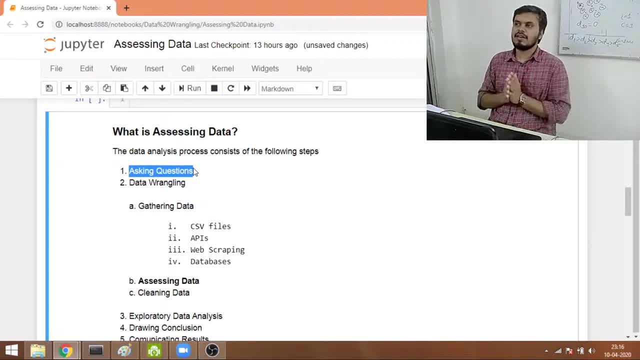 it's a talent, or it's a gift, or it's an art to look at the data and ask the right question right. and this, to be honest, no one can teach you. it comes from within. you will learn while doing it, or you are working in a domain- data- where you will automatically start understanding the question. 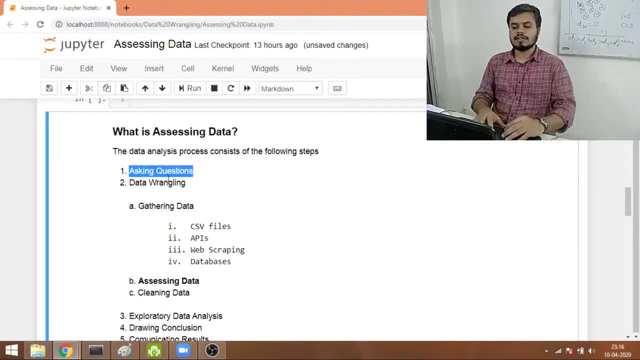 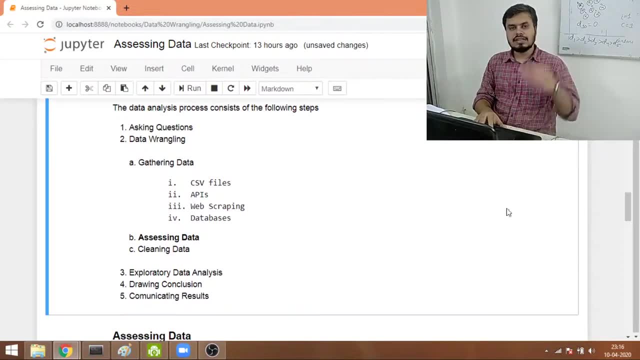 so we didn't work on this much. we went directly to the second step, which is data wrangling, and data wrangling is gathering data where you bring the data in. the first step is a very important step, jisme khud tin steps hota hai. so the first thing is gathering data where you bring the 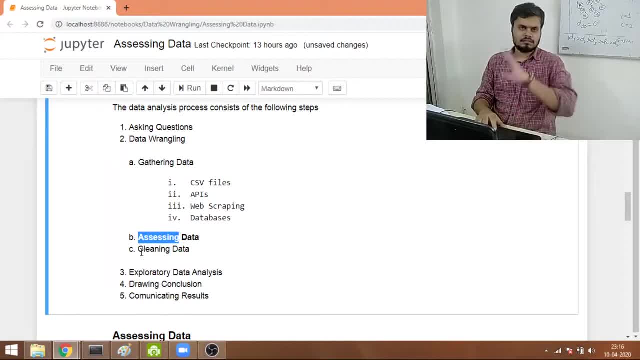 data. the second is assessing data. data ko ek baar dekhna, then cleaning data, unclean data ko thekh karna, and we know ki gathering data. it comes from various sources, so generally you will get a csv file from where you know you can directly analyze your data. but sometimes the data source is not. 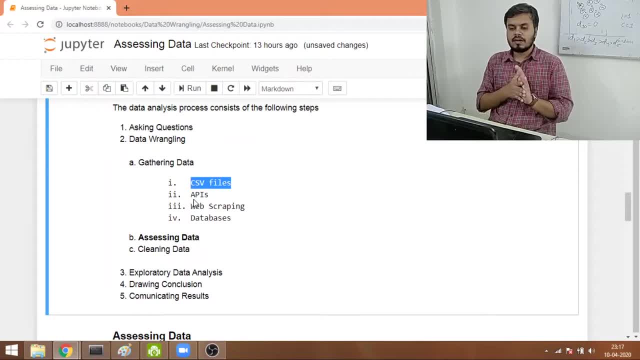 that case, you'll have to- you know- work a little extra in order to gather data. so there are three ways. the first one is API's- we have worked on it. web scraping- again we have worked on it. and databases- we have worked on it as well. and after that, 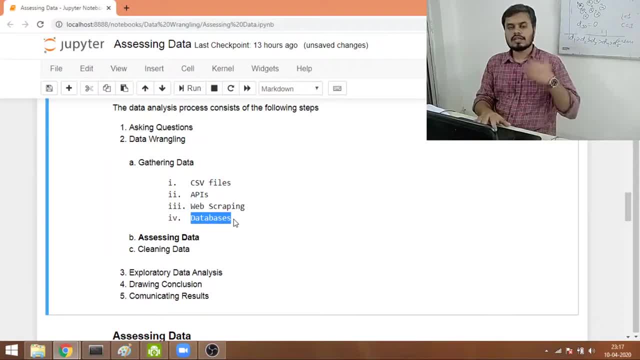 when you get the data, then now you assess the data so that you know where there are mistakes, and then you clean the data. whatever mistakes you have, you correct them. and the fourth step is exploratory data analysis, then drawing conclusion and finally communicating result. okay, so this video, this specific video, is dedicated to the second step. 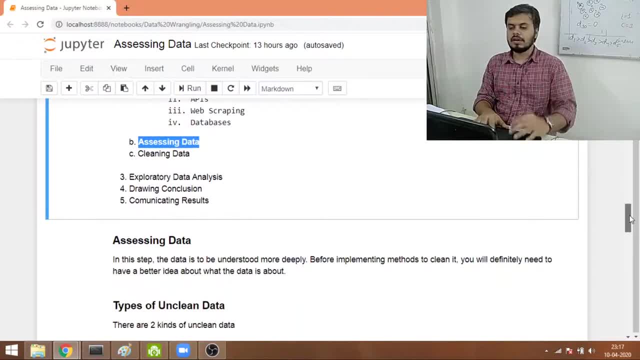 assessing data. okay, so assessing data is this step where the data- in this step, the data- is to be understood more deeply before implementing methods to clean it. okay, you will definitely need to have a better idea about what the data is about. simply speaking, you have to clean the data before you give it in the algorithm right and data cleaning. 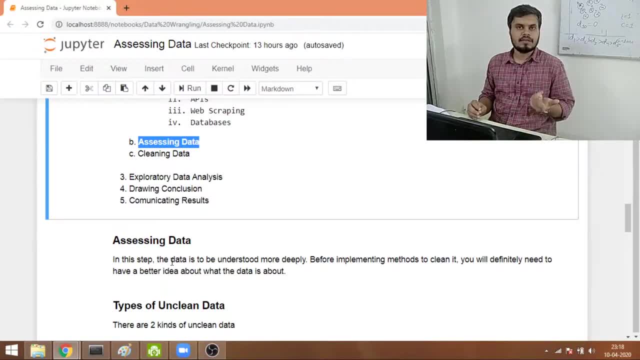 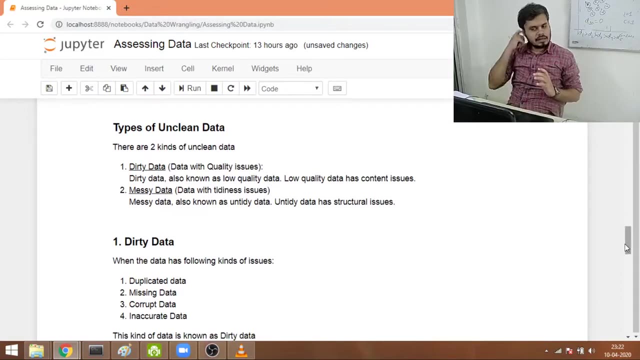 will be done only when you know where the issues are. so the process of finding the mistakes- we call this the assessing data. that's it simple, okay. so to clean the data, you'll have to first find out where the unclean data is and to find out 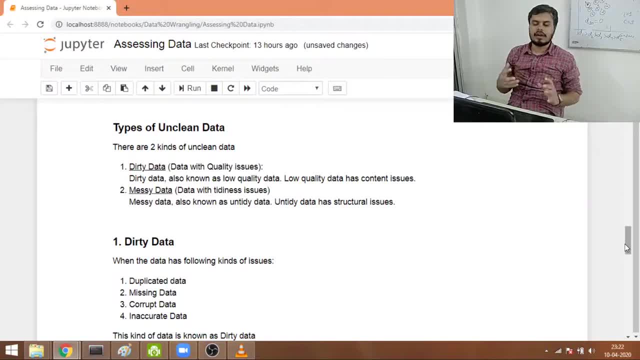 unclean data. let us first define what is unclean data. so, guys, first of all, this is not science. what we are studying is not science. nothing is defined means different data. scientists, data analyst work with different styles, so I am just trying to set in a framework. so 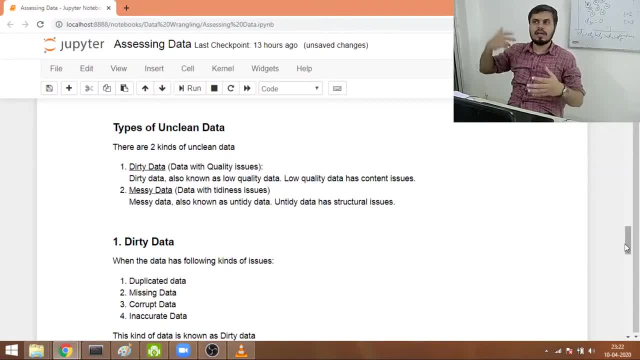 that when you get into this process, you remember that these are the steps. by roughly following these steps, we can reach somewhere. so unclean data is of two types. the first one is dirty data data with quality issues, and the second one is messy data data with tidiness issues. 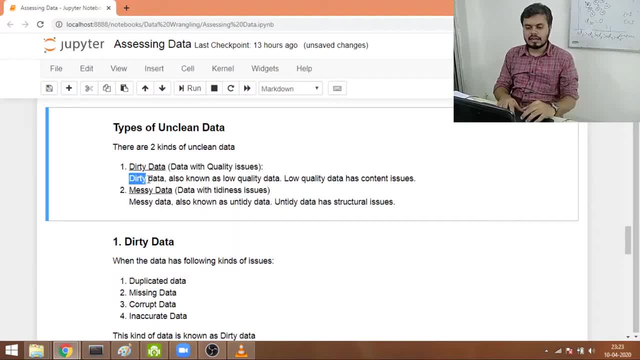 I will define what both of them are. so dirty data, also known as low quality data, is a data which has content. issues means there is a problem in the content of that data, so we call it dirty data. second one is messy data, which we also call untidy data, and the problem 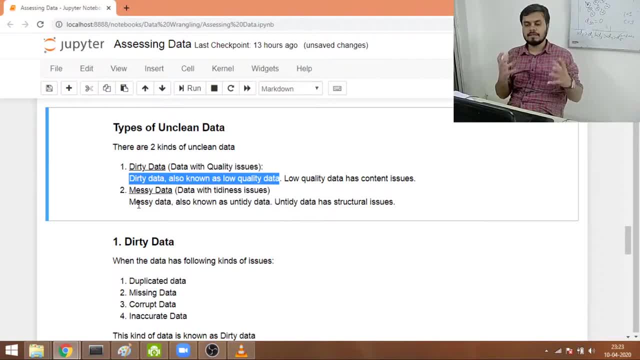 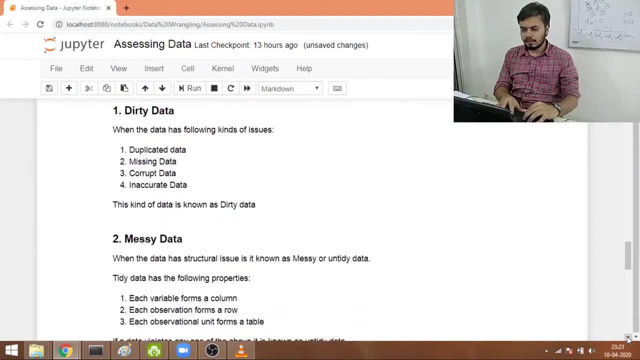 of untidy data is that it has structural issues. I will explain both better. so let me first explain what is dirty data. so dirty data is a data when the data has following kind of issues. so one issue may be that it has duplicated entries. that makes the data dirty. 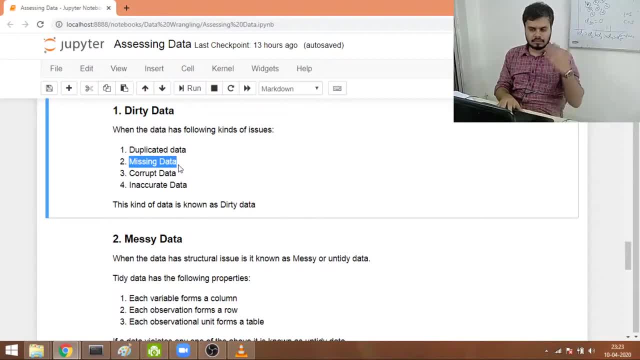 data: Ok. The second is: missing values. are there? again, one major issue. third, data is correct. you are not able to see what is there in the data, or inaccurate data- ok, there is a problem in the accuracy of the data. you are able to see that it is not correct, ok. so if you 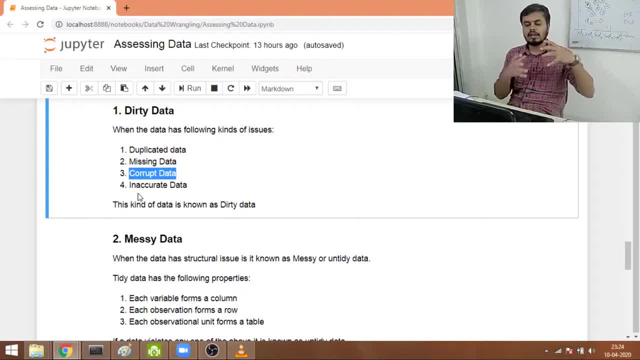 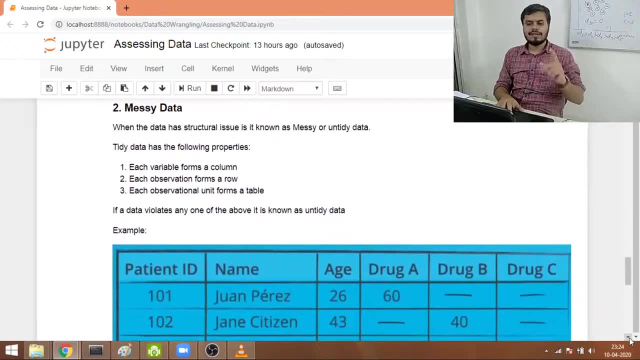 are getting these four types of issues in the data, then this data is called dirty data. ok, Second, let's define what is messy data. so when the data has structural issues, it is known as messy or untidy data. see what Subtle data is. will read its definition. 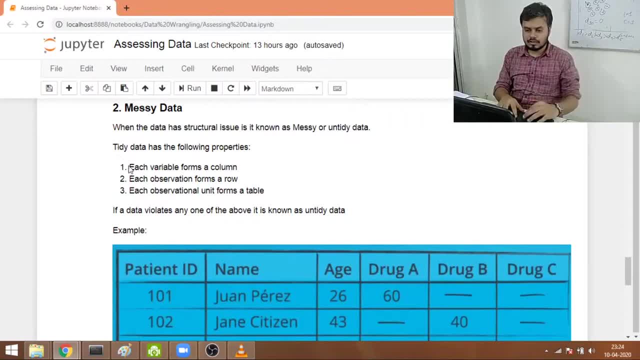 So the rule of tied data is the first rule is: each variable forms a column. this is the first rule. each observation forms a row. This is the second rule. The third rule is: each observational unit forms a table. if any rule is getting violated, 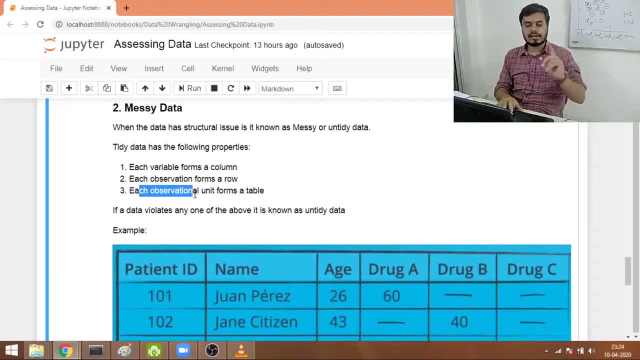 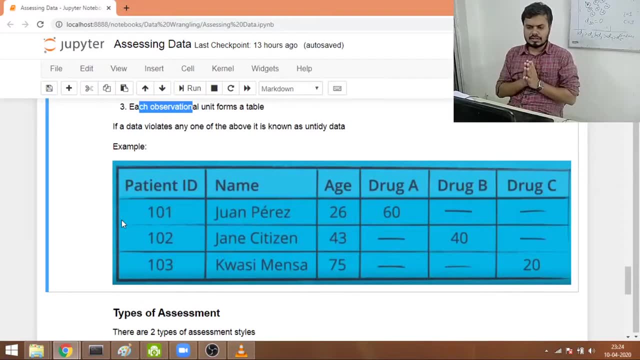 from in all the three, then it will become messy data or untidy data. I will show you one example. ok, notice this. here we are keeping the record of the patient and giving him some medicine. this is his record. now, what happened here is that we should have only one drug column. 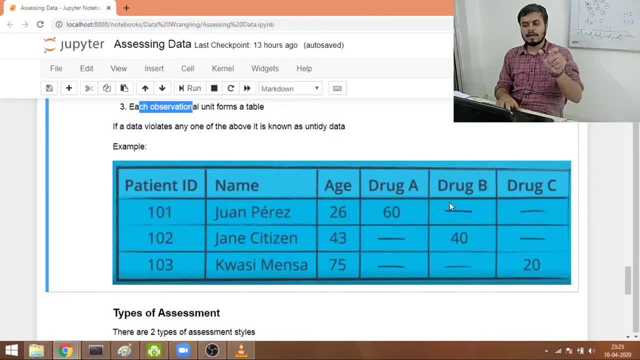 and its dose. but we made three columns, one specifically for drug A and one for drug B and one for drug C, and you can see that the patient is either taking drug A or B or C. this means that the table that is being formed is very sparse, meaning that many nan values will come. 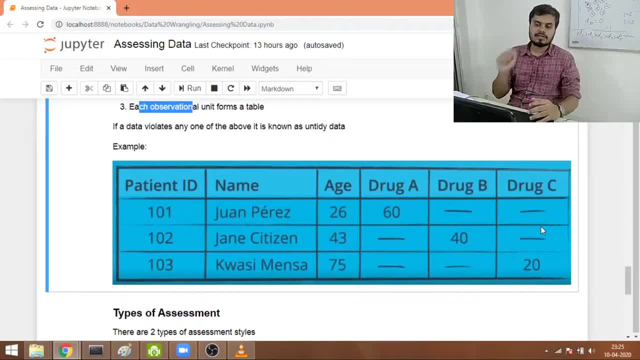 now, this is a structural issue and because of this this data set becomes untidy and messy data. so I hope the concept of unclean data is clear. I am summarizing it once: unclean data is of two types. so there is dirty data, which has quality issues, and second is messy data, which has structural issues. 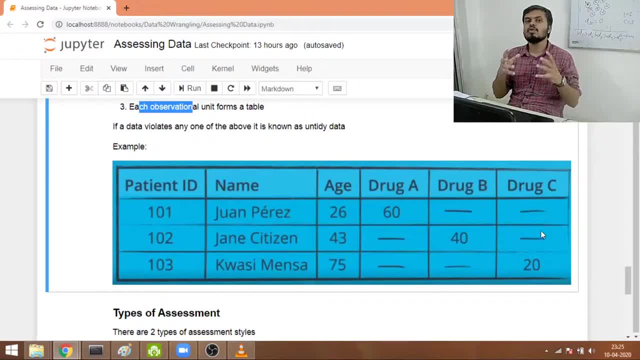 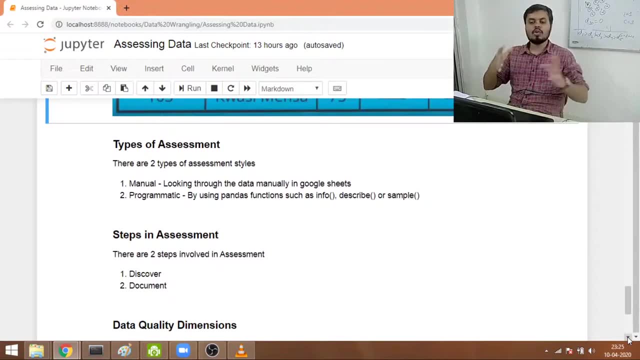 you have to find these two types of things. ok, now, to find this, you have two options. there are two ways to find this. ok, so there are two kinds of assessments that you can do. the first one is manual assessment, where what you do is you just look upon the code and you try to find out the patterns. 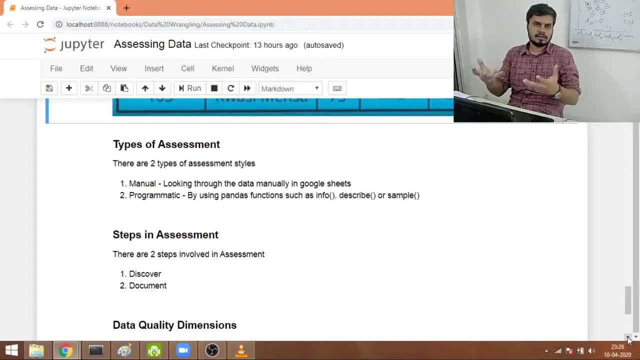 or you know, you try to find out these kind of anomalies, you try to see these errors directly with your eyes. ok, no programming tools, no functions, nothing. the data is there and I am looking at it manually. ok, there is not much benefit, to be honest. 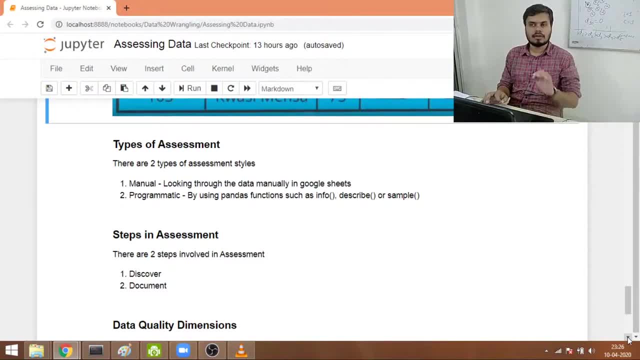 but one major benefit of manually checking is that you start getting a very clear idea of the data guys. you won't believe all the good students I have seen whose data analysis is very strong. I have always noticed a common pattern in them: that they look at the data for hours. 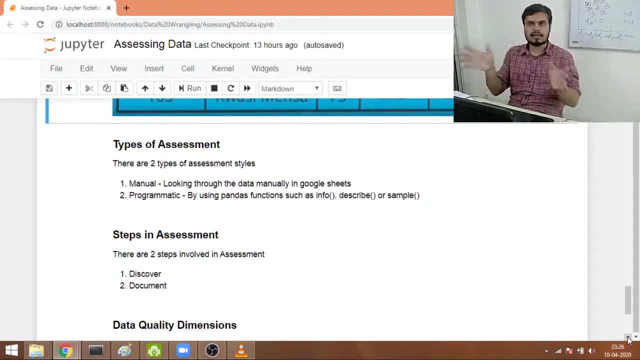 meaning they are looking at the data on the screen. they are just looking at the data, nothing. they are not even asking questions, they are just seeing data. so they are actually filling their subconscious mind with that data, right? so this should be done. ok, so manual assessment is the first assessment type. 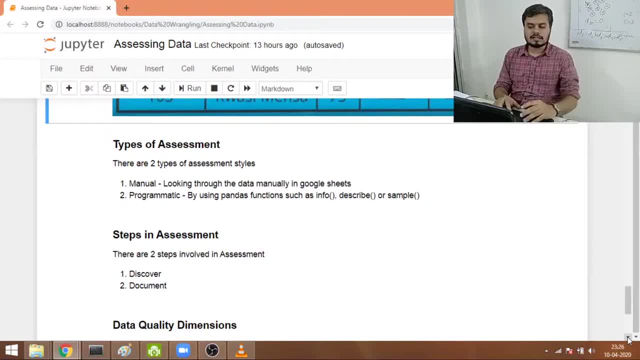 where you are looking at the data directly- ok. the second assessment is programmatic: ok, where you use the functions of pandas- info function, describe function or sample function- ok- and you look for those errors in the data- ok. so you are doing the assessment in two ways. 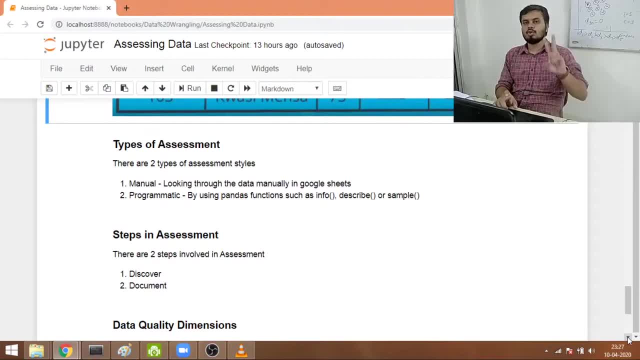 second, when you are doing these assessments, you have to follow two steps. first step: you discover these errors, these anomalies. ok, this is the first step. obviously, in assessment, the first step is to discover and the second, very important step is to document it, meaning you have to think and see. 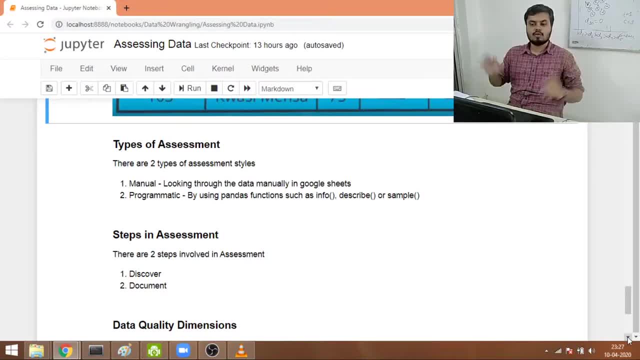 and understand that there is no error here. you have to note it down somewhere so that when you go to clean you have a proper documented record that I have to correct this, then I have to correct this, then I have to correct this. ok, so you have to follow a process. 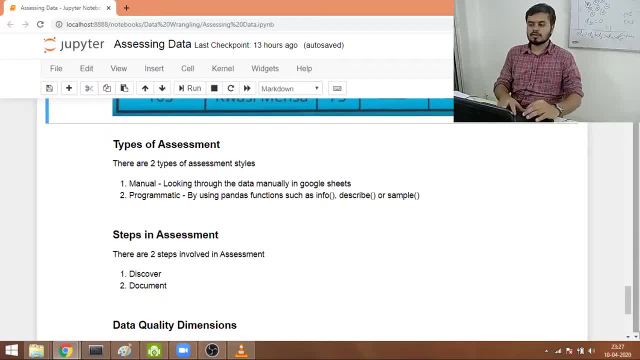 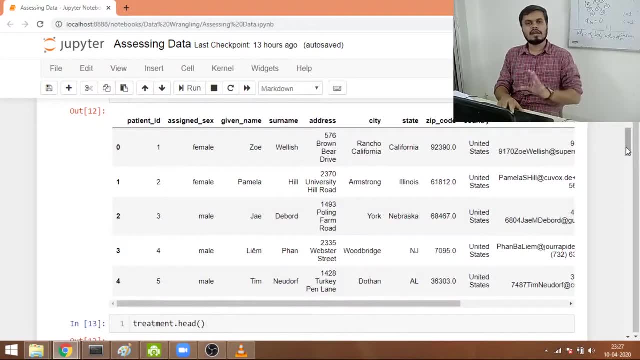 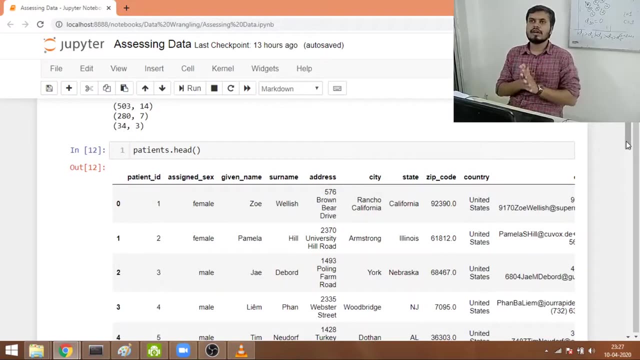 ok, so this is what we will do in this video. so what we will do is I have some data here and these are toy data sets, meaning whoever has created this has deliberately left some errors in it, and this data is clinical trial data of insulin. ok, so if you know about insulin, 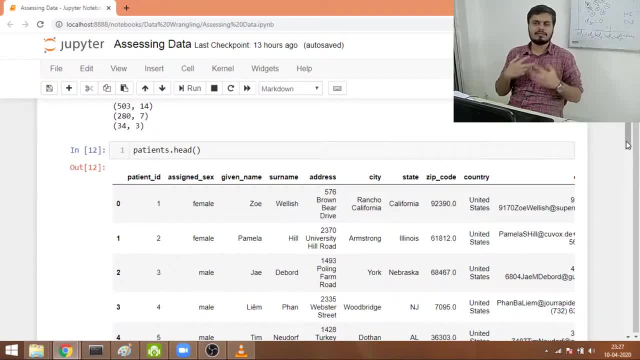 it is used to- I don't know- to reduce diabetes and all. I don't have much knowledge about it, but insulin is used for the cure of diabetes and insulin generally. there are shots of insulin, there are injections, so these people have maybe taken some medicine so that you can take that medicine. 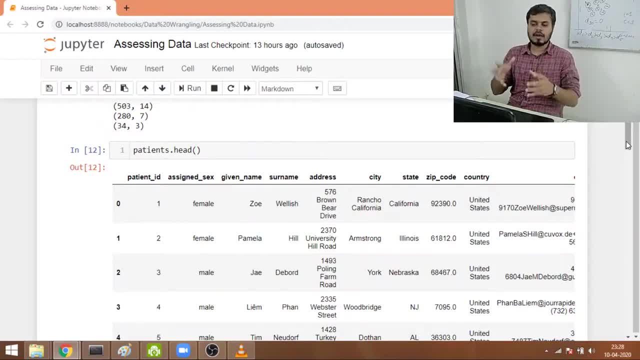 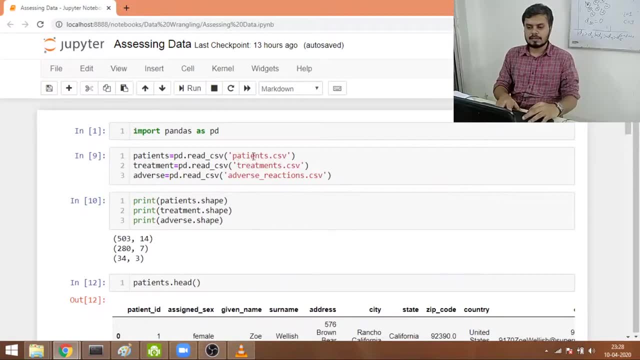 rather than taking shots. so these are some patients who are trying it and this is the data of that. so here we have three tables. so the first table is patientscsv, the second table is treatmentscsv and the third table is adverse reactionscsv. ok, I have taken out the shape of all three. 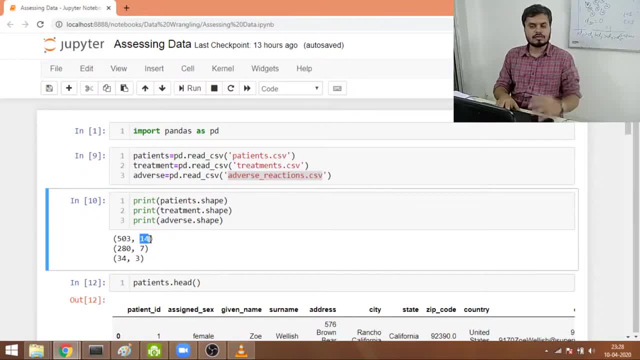 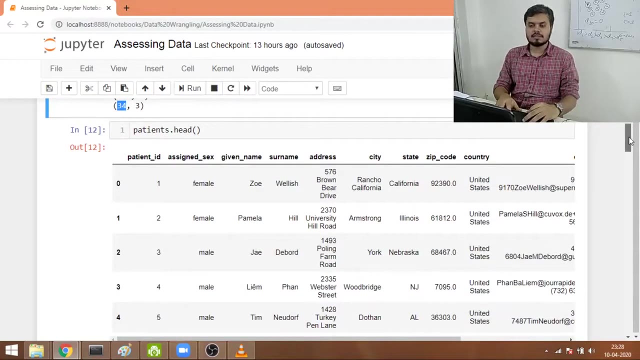 so there are 503 patients in patients and there are 14 columns of information, and in treatments there are 280 rows with 7 columns, and in adverse reactions there are only 34 rows. ok, and here are all the data frames. this is patients, this is head. 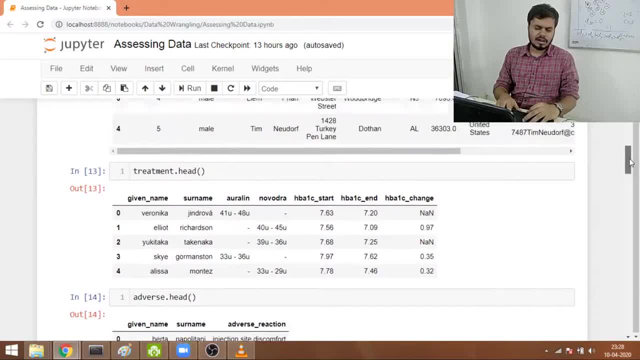 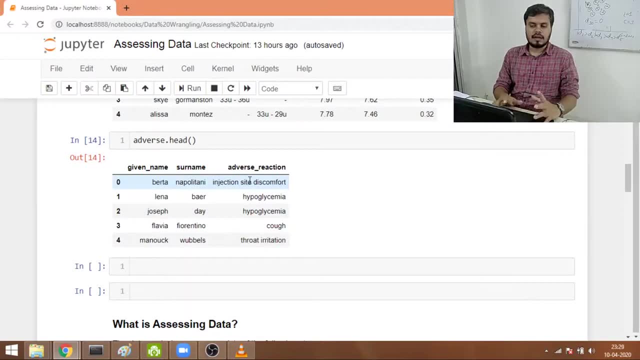 and sorry, I am not. I am sorry, this is not head, this is treatments and then this is adverse reactions. ok, so we have these three now. what is our goal in this video? that we, through manual assessment and programmatic assessment, through both types of data issues, means. 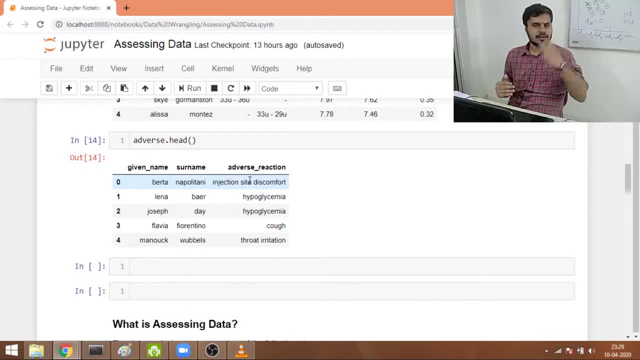 unclean data we will fetch or discover. the first one would be dirty data with quality issues, and then we will also try to find out untidy data or messy data with structural issues. ok, so that is the goal of this video. ok, guys. so now our next goal is: 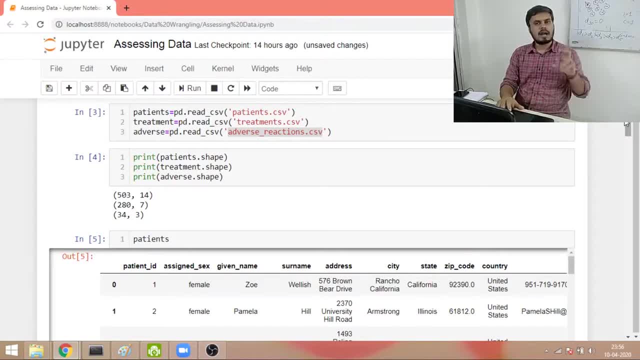 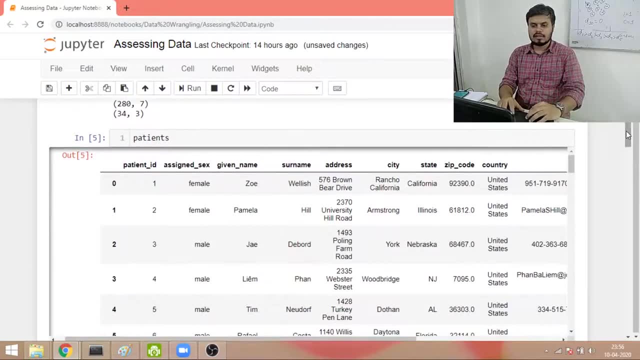 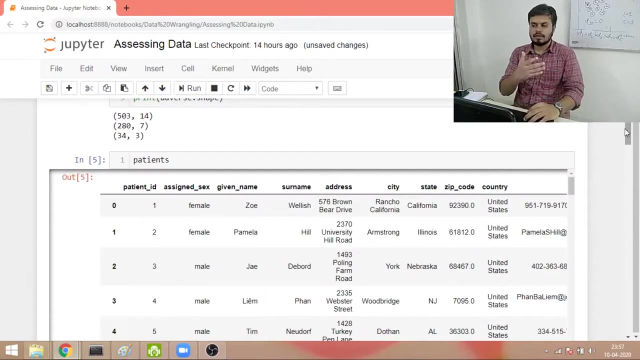 our next goal is to do a manual assessment and find quality issues in our data. ok, so I have loaded all the files- patients, treatments and adverse- before going forward. see, the idea of manual assessment is that you understand the data first of all, because that is very, very important. 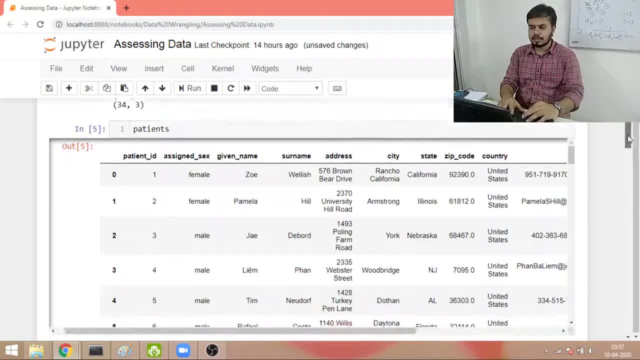 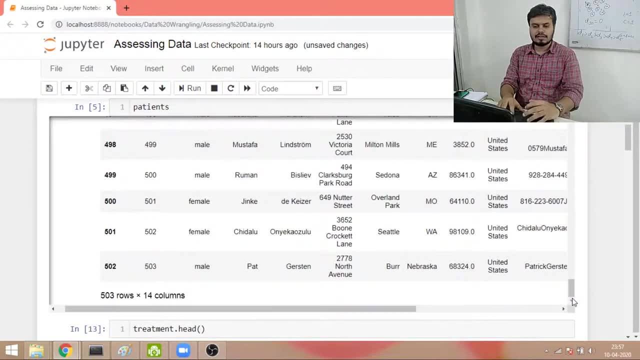 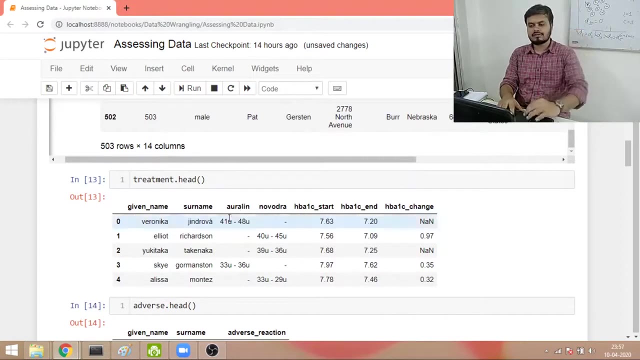 you should understand the data. like one thing. I forgot to tell you what happened here, that these are all our patients. so there are in total 503 patients and we have on them. there are two ways of giving insulin. the first one is this, Novotra, where you put injections. 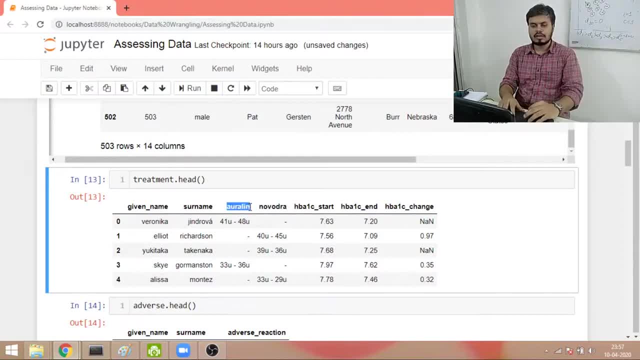 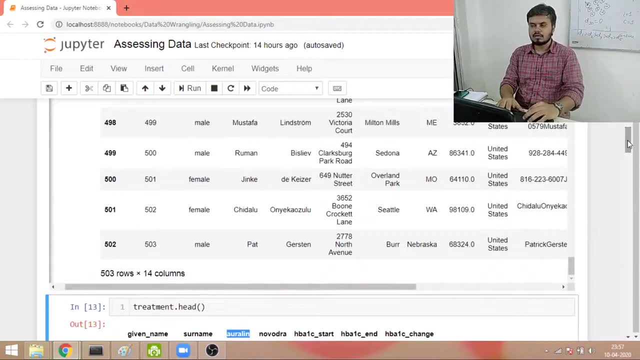 in the patient's body. and the second one is this New Auralin oral insulin, where insulin is given through medicine. ok, so what happened here? in this data set, out of these 503 patients, 175 patients were taken. actually, 350 patients were taken, 175 were given Novotra. 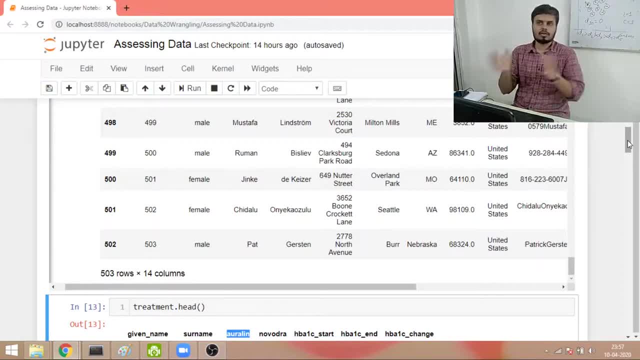 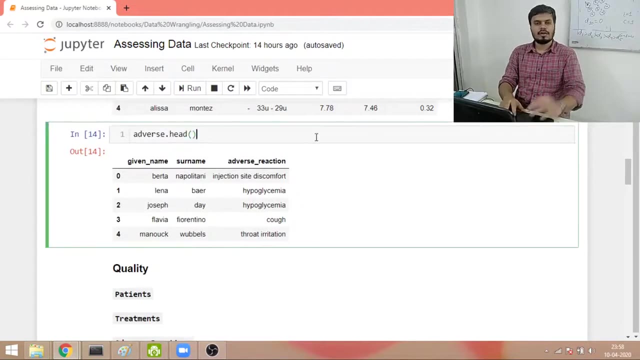 and 175 were given Auralin. ok, and both were compared side by side. that the impact of Novotra, of the injections, is the same impact of your medicine or not. that's the whole idea. ok, and then those people who got some adverse effects. that data. 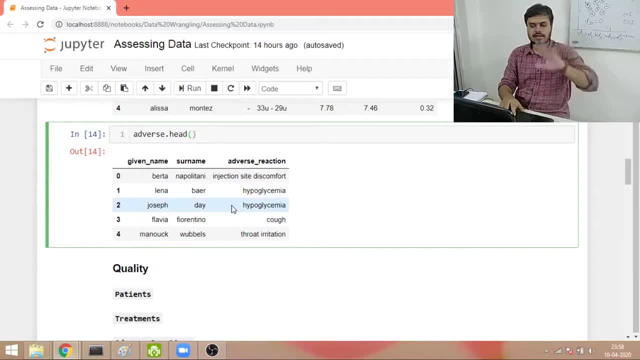 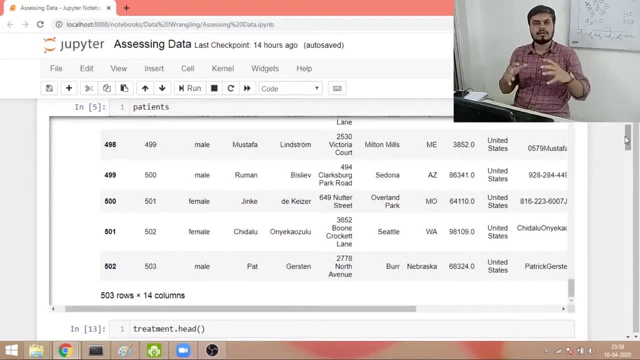 we have put in the adverse reaction table in the third one. ok, now what we have to do is we will do a manual assessment of all three data frames and we will try to find out what are the problems- quality related issues- which are in our data set. 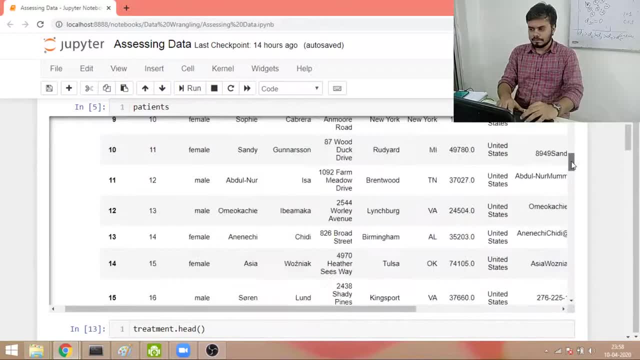 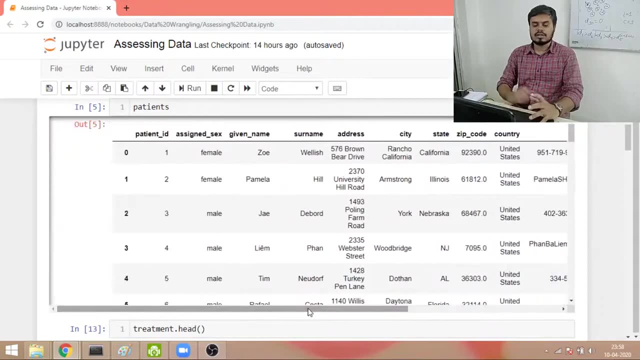 ok, so this is the first one. patients now see what should be the starting point: that you focus on the thing which is most important in your data. ok, so for us the most important thing is this: in the treatment table, this particular column is the most important column. 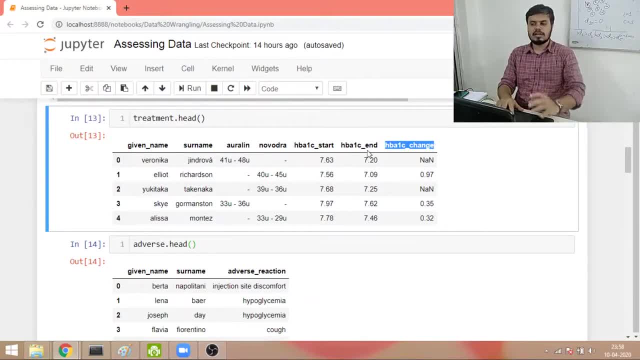 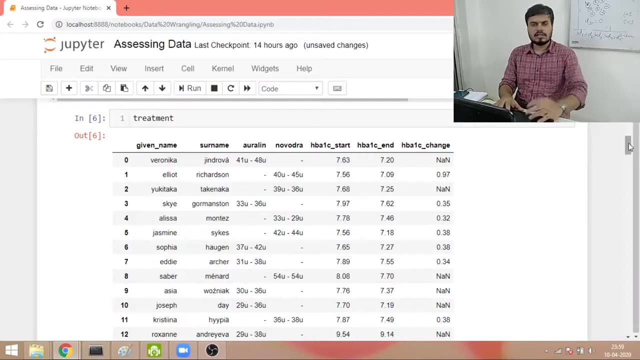 HBA1C change. ok, from this change you will get to know that Novotra and Auralin, these two ways of giving insulin, are equally effective or not. ok, so if I run the treatment table completely so directly, I can see that my most important column 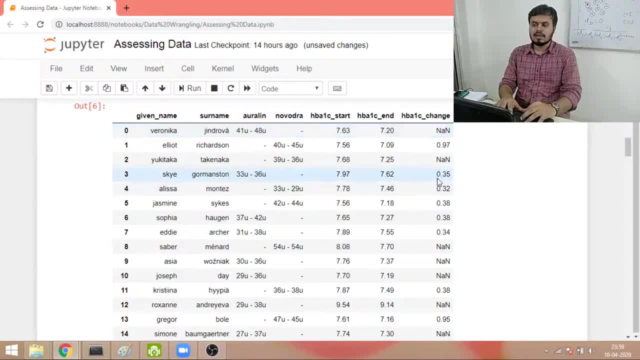 HBA1C column. here is the most important column. here there are many missing values. now how does this come out? H1 HBA1C change comes out HBA1C start minus HBA1C end subtract. and what happened here? I don't know. 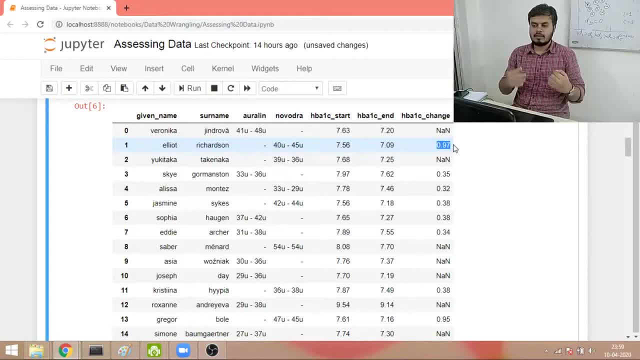 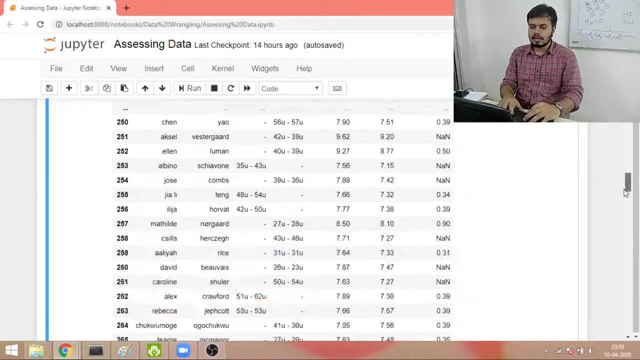 whoever created the data. he in some subtraction, in some he forgot to do or he skipped, whatever the reason. but because of that we have many new values. ok, so this clear cut. I have the first indication that there are some quality related issues. ok, so what we have to do? 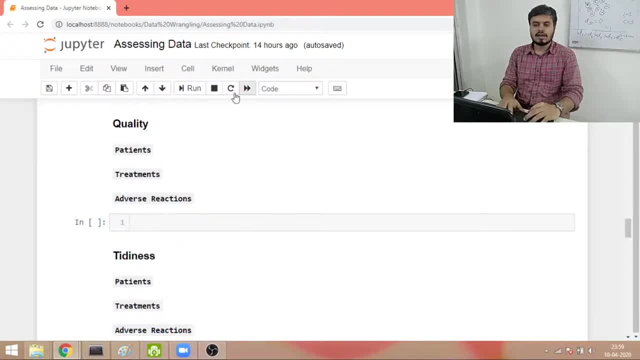 by going down. what I have done is I have made two cells: one in which I will write quality related issues for all of three tables- patients, treatments and adverse reactions- and similarly, I have made one more cell where I will write tidiness related issues for both patients. 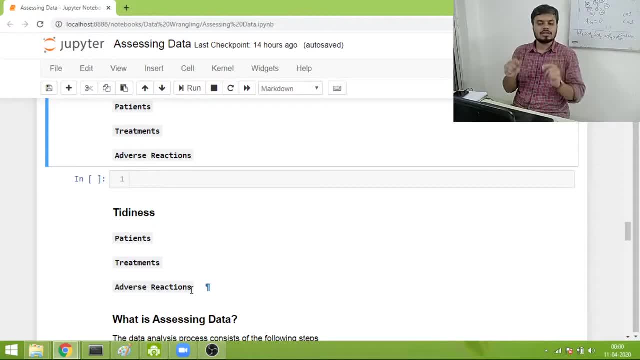 and treatments and adverse reactions. ok, now, the whole idea of doing this thing is because I told you first, you discover- because when you go to clean you will have these two cells, you will have a target- that I have to do this. ok, that's why we are doing. 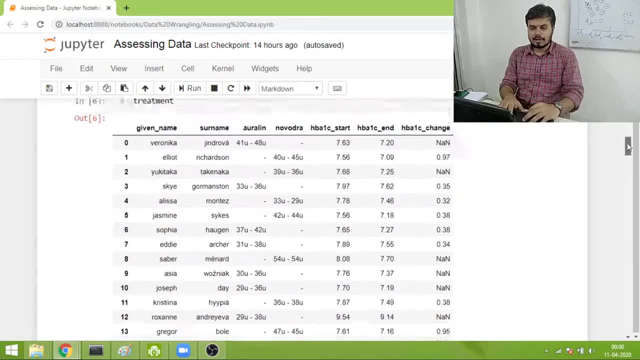 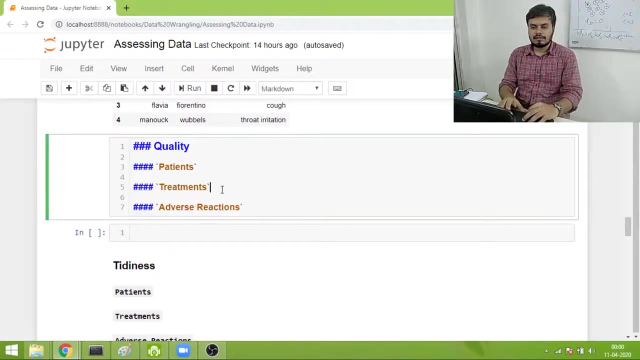 this documentation. so now we can clearly see that in our treatments table in our treatment table, this column HBA1C change has missing values. so what we will do, we will quickly go and document this. ok, so we will go to quality and inside treatments table I will add: 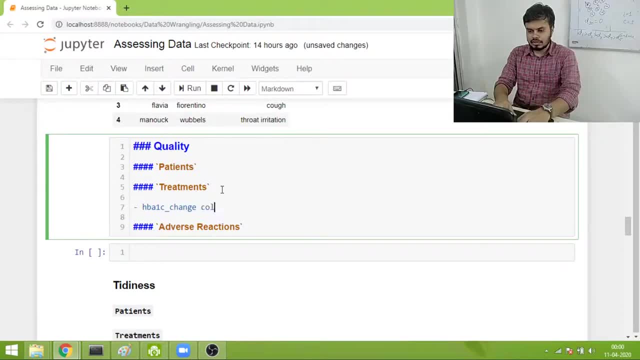 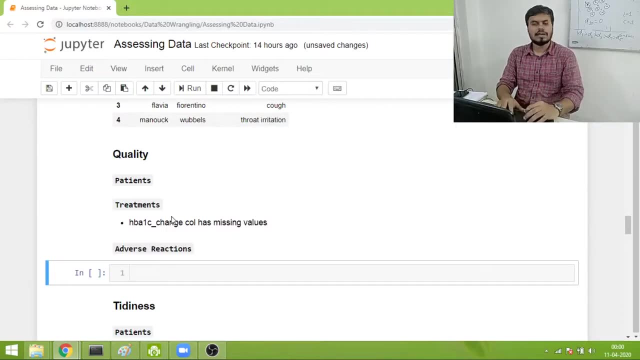 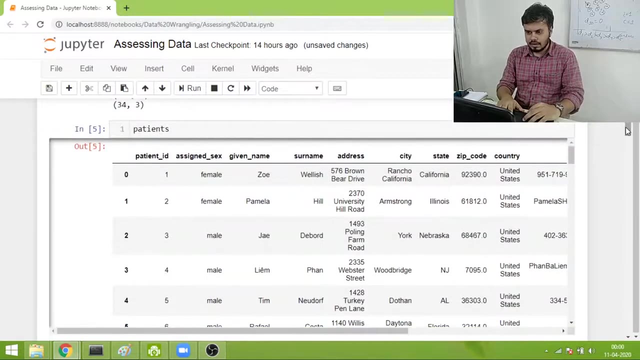 H1B2- H1BAC- change column has missing values. ok, this is my first thing. ok, now let's try a little more to explore like: this is patient's column here, if you try to scroll or if you try to see the various columns. so 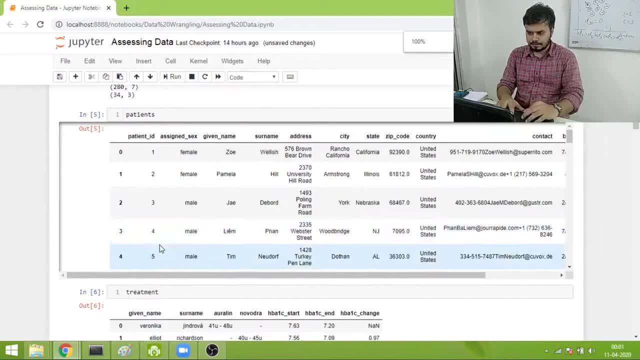 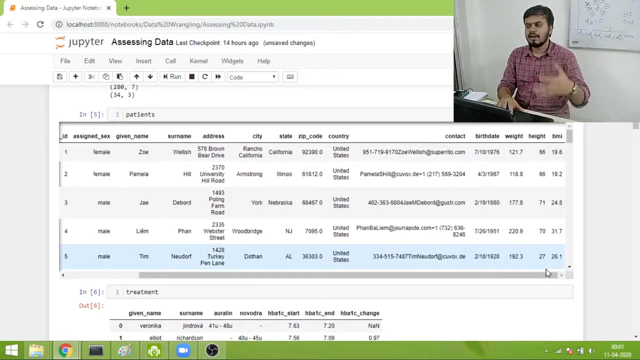 I am zooming in so that you can see. yeah, so here there is only record of patients. so sex name, surname, address, city, state, zip code, country, contact, birth rate, weight, height, BMI. ok, here you can see one error that we have somehow represented zip code. this column is: 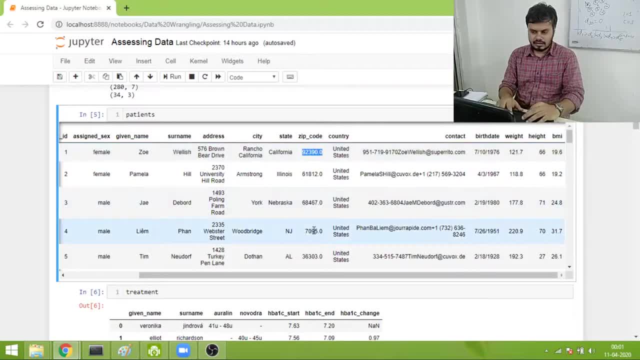 a decimal right. one more clear cut in the first 5 rows. I can see in the first 5-6 rows that some zip codes are of 5 digits and some zip codes are of 4 digits. zip codes should be consistent, means should be of 5 digits. 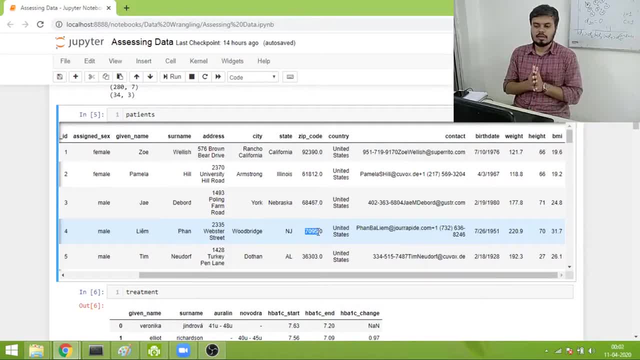 like in India. maybe not in India they are of 6 digits. in US I guess they are of 5 digits, but here there are certain zip codes which are of 4 digits. first is that zip code is represented in decimal, which should not be. it should be a character. 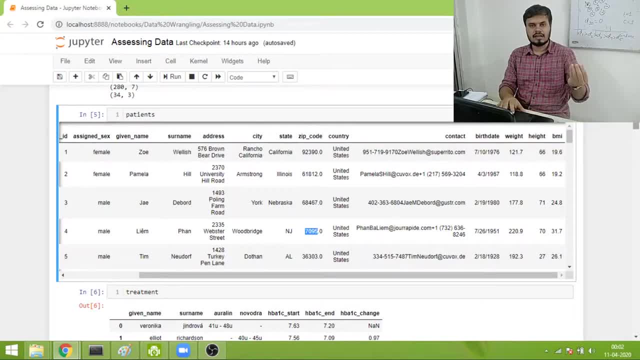 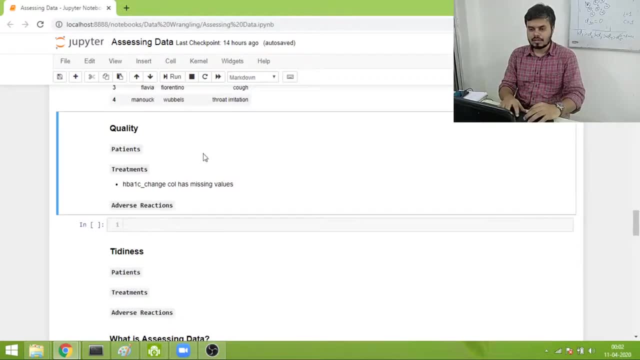 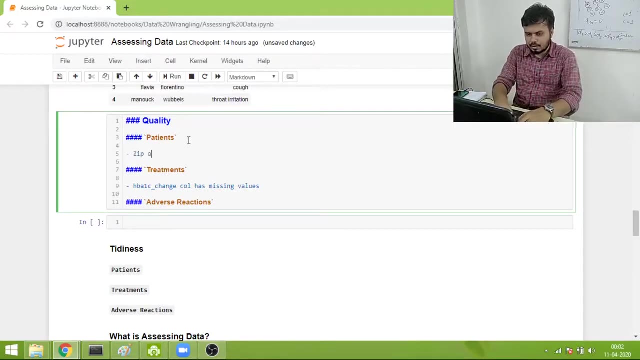 or a string. second, some zip codes are wrong because one digit is less ok. so what we will do, we will document it by going down. so we will go to patients column and we will write. the first thing that we will write is zip code. column is a. 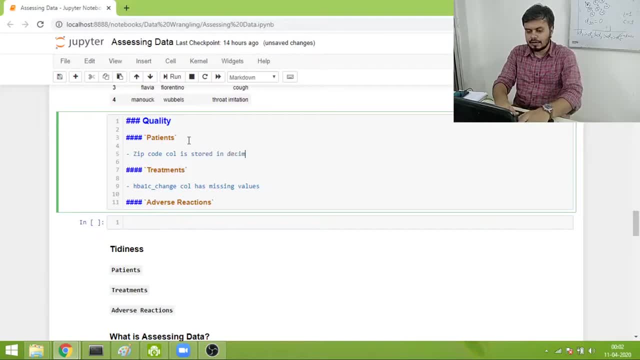 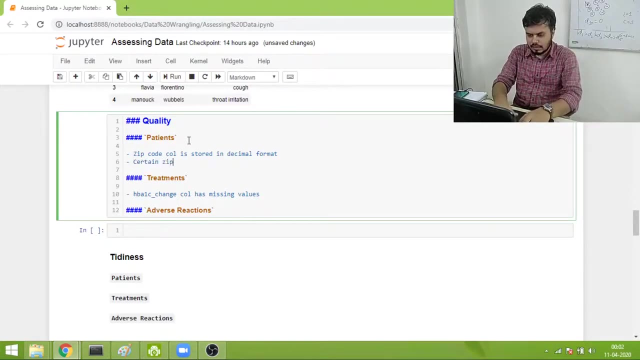 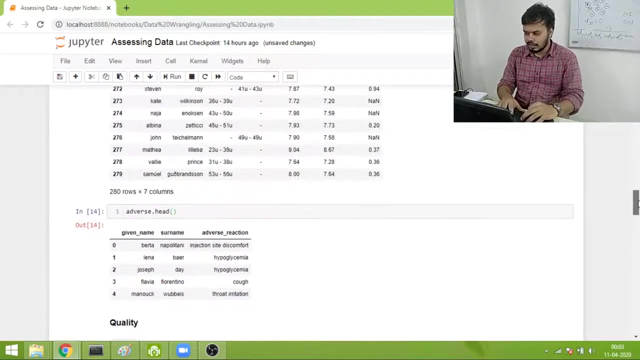 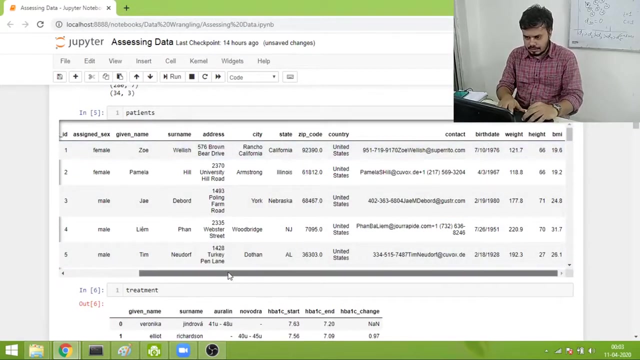 stored in decimal format. ok, we are just writing this. second, we are writing: certain zip codes are of 4 digits. right, we have run this, that is it. we have done this, that is it done. now we are looking at something else like: ok, one more thing I noticed. 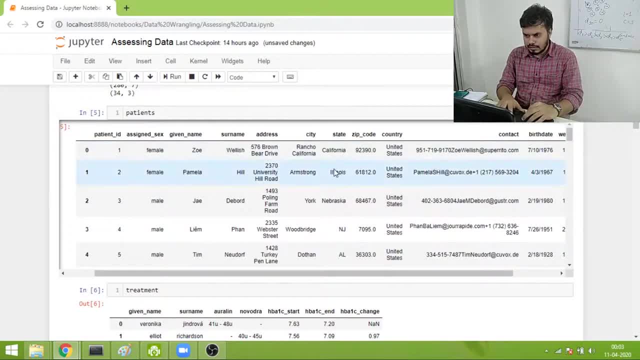 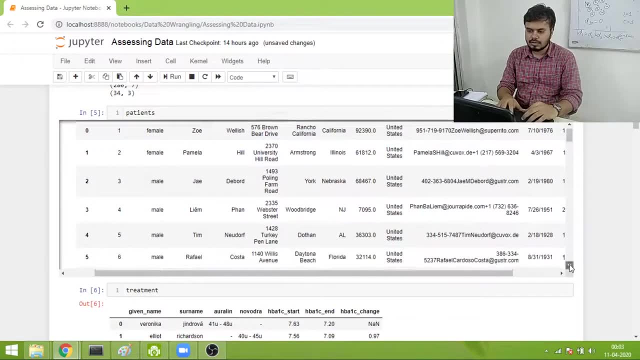 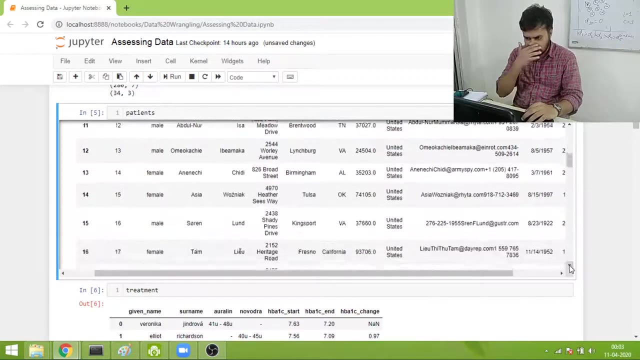 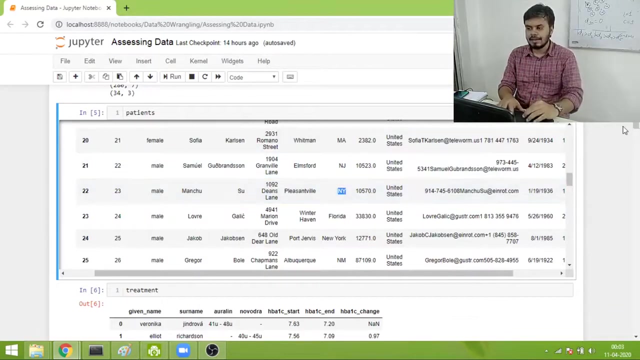 here. that is that states. you know, sometimes they wrote full name to encode states and sometimes used abbreviation, short form. ok, I will show you like. they used New York and Hawaii. so, in consistency, the problem is data. ok, so we are documenting this, we are going down and here. 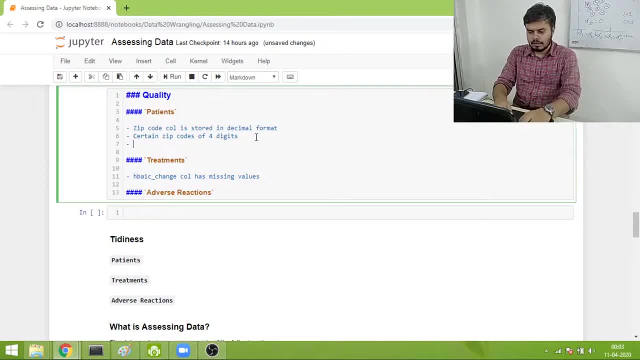 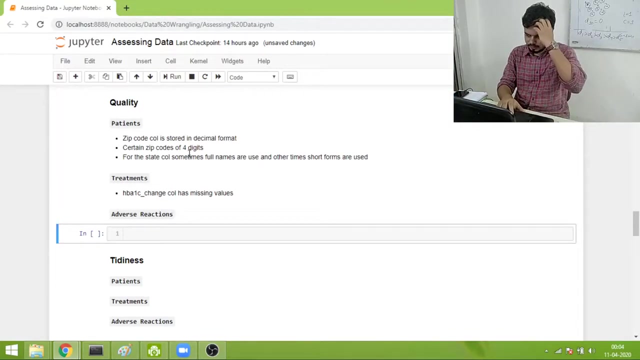 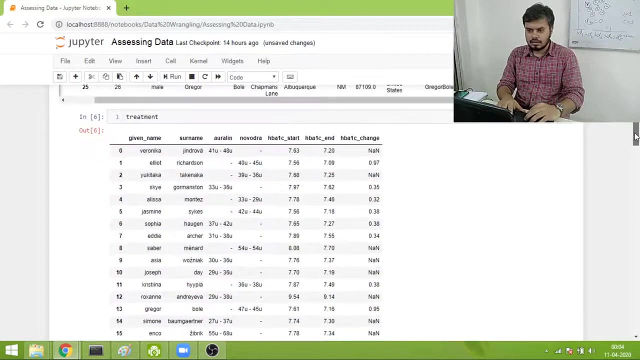 we are writing in the patients table for the state column. sometimes full names are used and other times short forms are used. short forms are used. ok, this is done. third, our quality related issue. next, what we will do is ok. now let's focus on this column. let's focus on 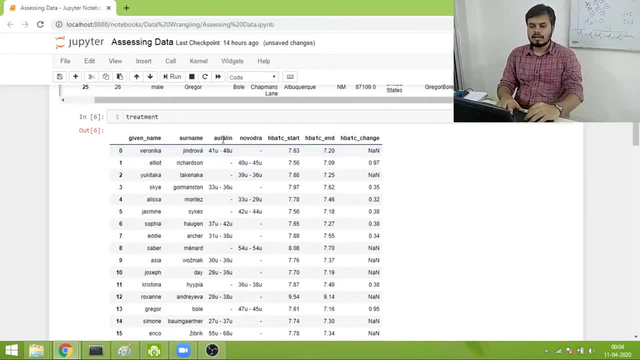 treatment data frame. what is here that, if you notice this is about the dose: lower 41 u u, as in some unit, and 48 is the highest for this patient and similarly in novodra same. they have followed the format. so first of all, this is not looking. 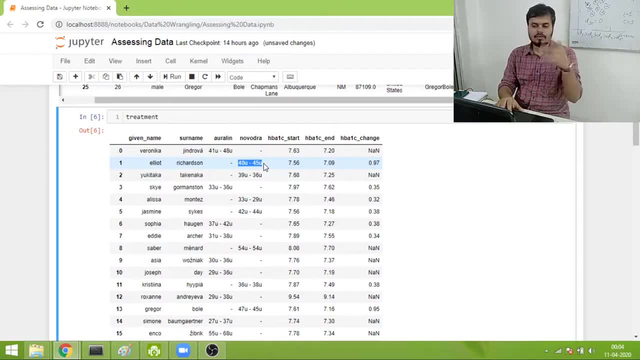 good structural changes. structural issues are seen, but we will cover that on tidy data time. but for now, one major issue is that, since these things are number, dose how much this is number, which is why this whole column has become string and it will be difficult to do mathematical. 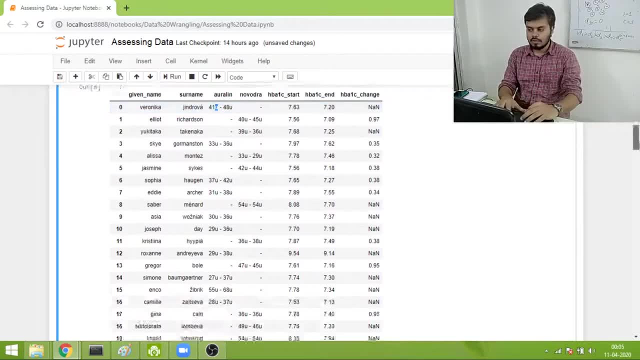 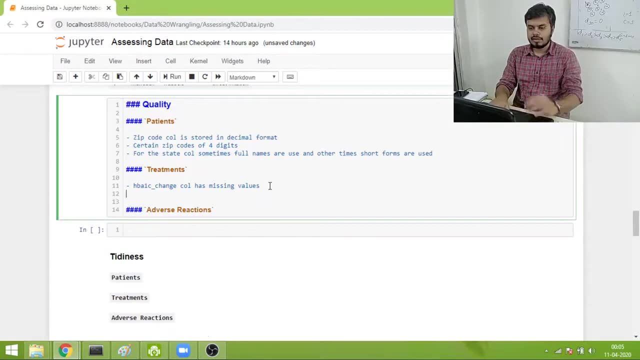 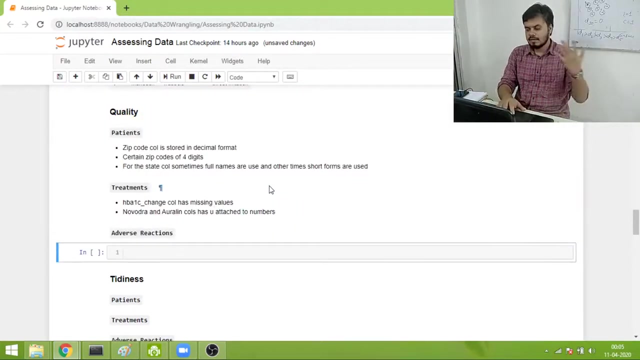 calculations or comparisons on it. so we are also documenting this. we will write inside quality, inside treatment. we will write that novodra and auralin columns has u attached to numbers. so this is one more issue that we want to solve. the next thing is: yeah. 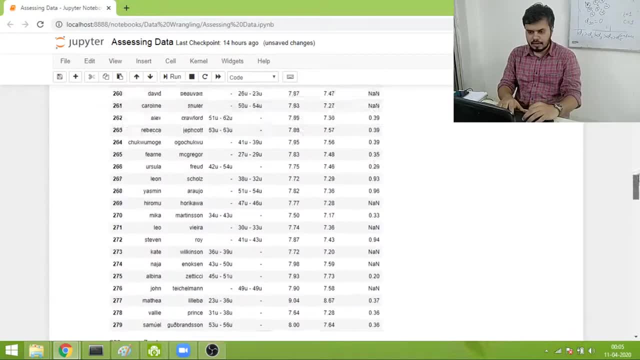 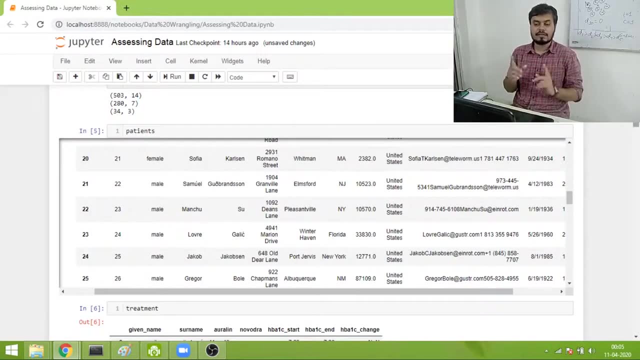 so i told you that there are 503 patients and out of those 503 patients we have chosen 175 plus 175 patients: 175 with novodra, 175 with auralin. but the problem is that when you look at this data, the treatment- 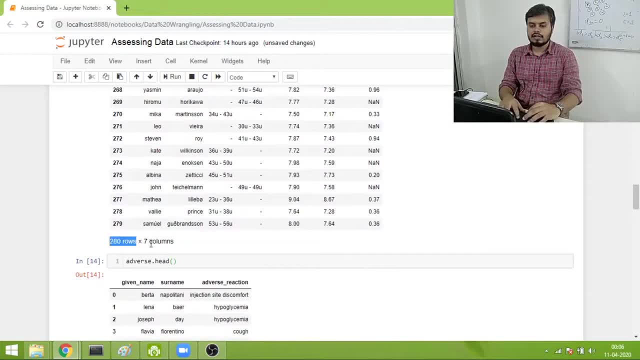 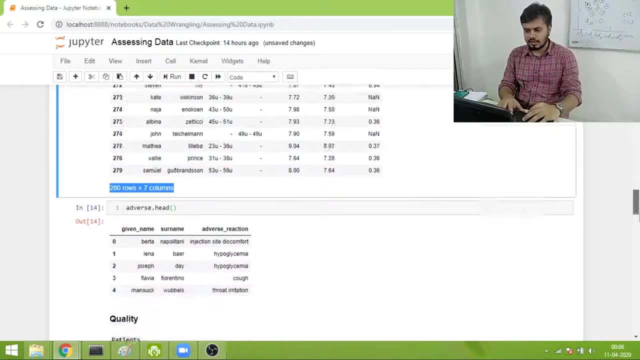 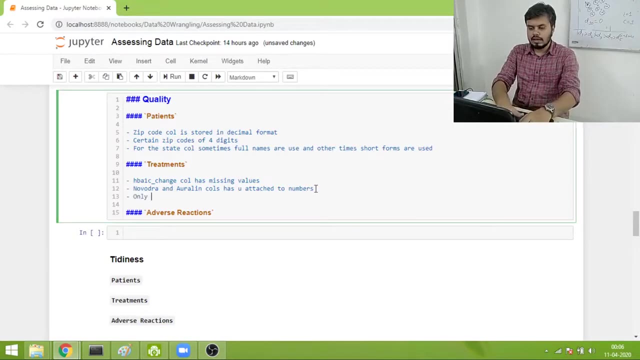 data. you will notice there are only 280 rows, so it should be 350, 175 plus 175, but there is only 280, so data is missing. so this is also a quality issue. so we will write in the treatments table: only 280 rows are. 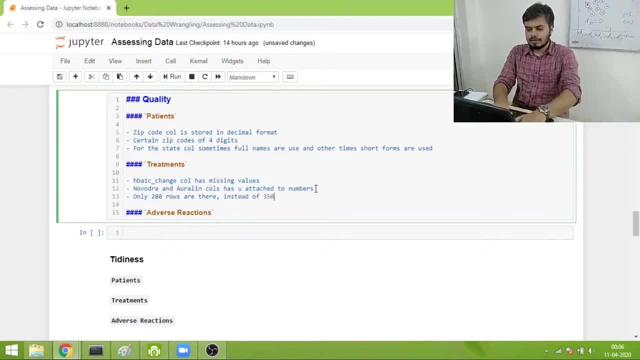 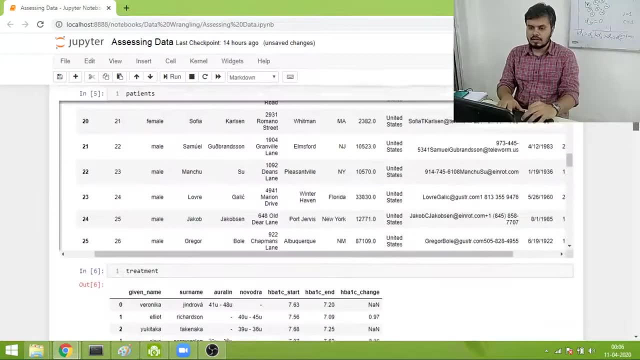 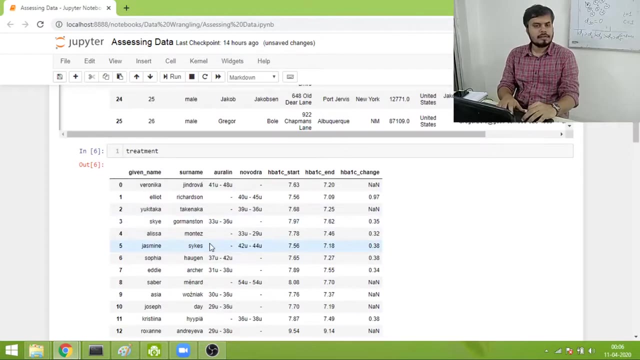 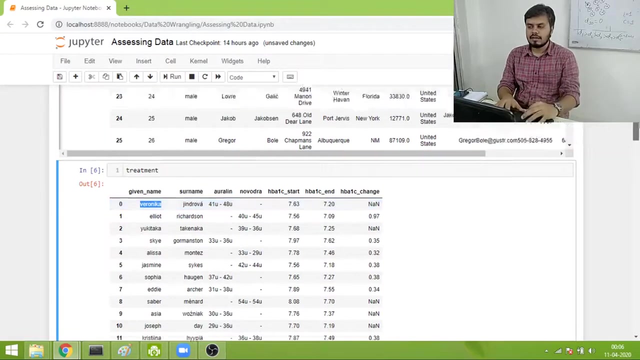 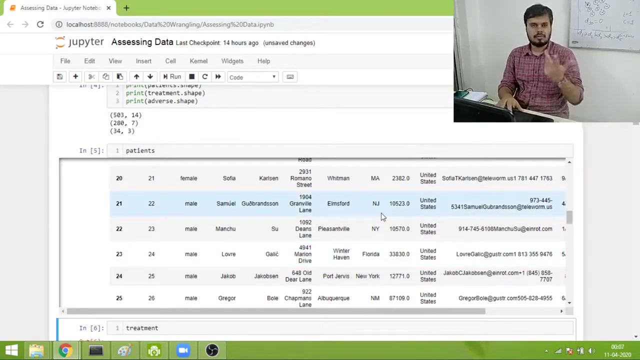 there instead of 350. okay, and finally, one last thing is that if you notice the patients here, some of these patients, we are bringing them to the treatment table, but here, if you see their name and surname are in small column, you will not be able to search. 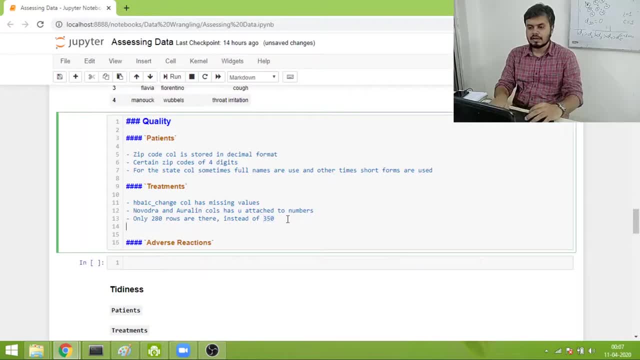 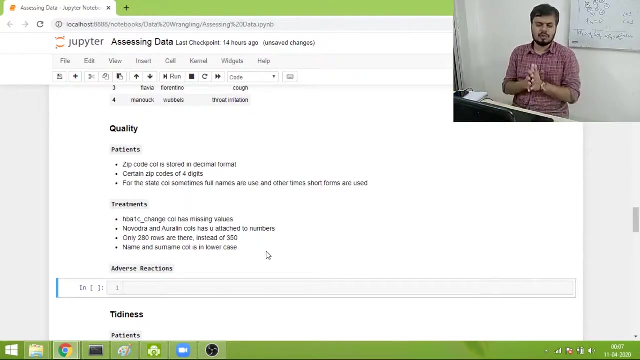 so we will write here in treatments: table name and surname. column has is in lower character, lower lower case. sorry, column is in lower case. so this is our case and this is our manual assessment. there are many more things. to be honest, people have made many mistakes in data. 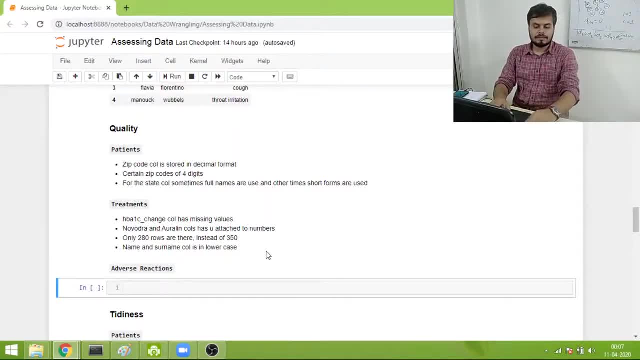 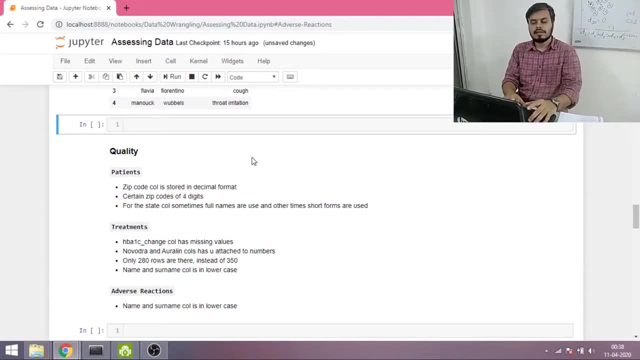 but I am just giving an example: how to do quality issues. okay, okay, guys. so next we will talk about data. okay, so simple meaning of programmatic assessment is you will use pandas functions. by using it you will get idea about complete data because, see in manual, you have to. 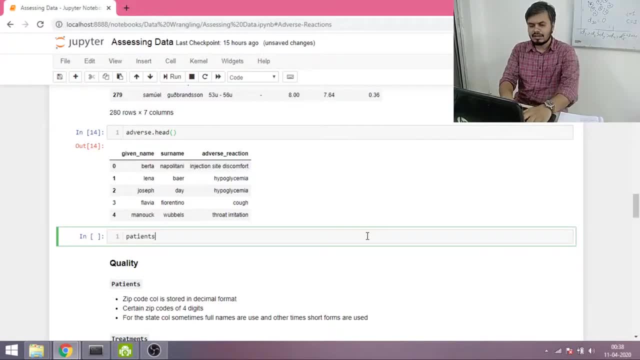 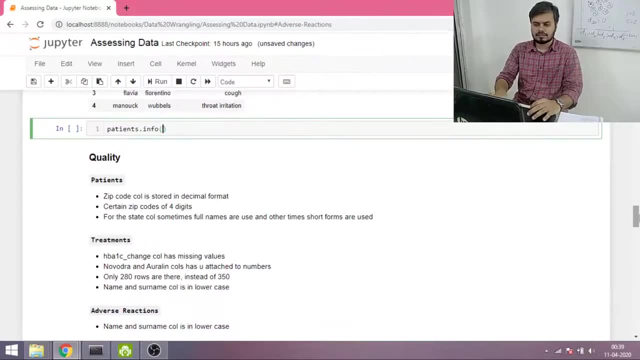 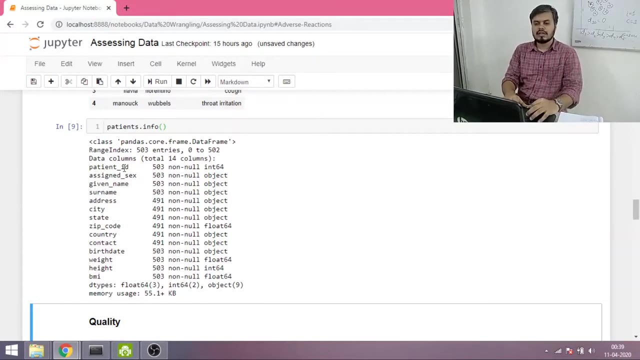 put info function on all data, without even thinking anything, on all data frames. I will show you so I put on patients and if you put info function on patients and how much data, memory, usage, things like that. now one thing is clearly visible: address, city, state, zip code. 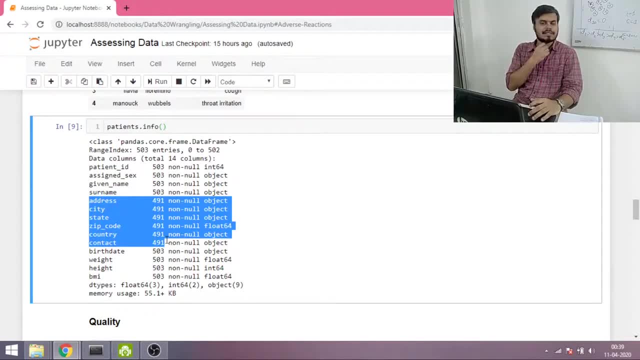 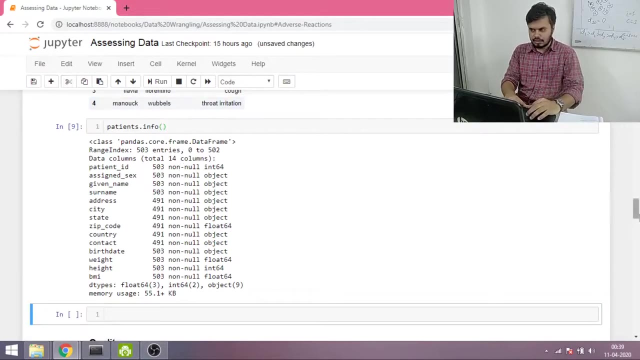 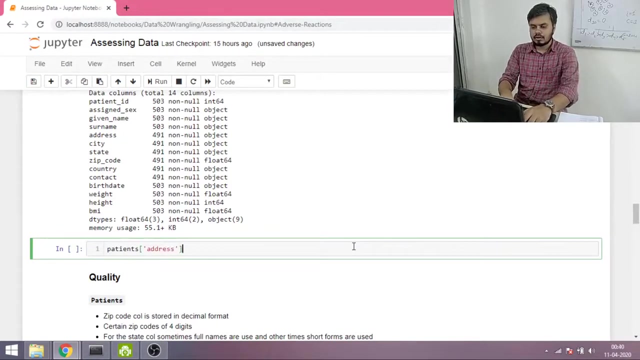 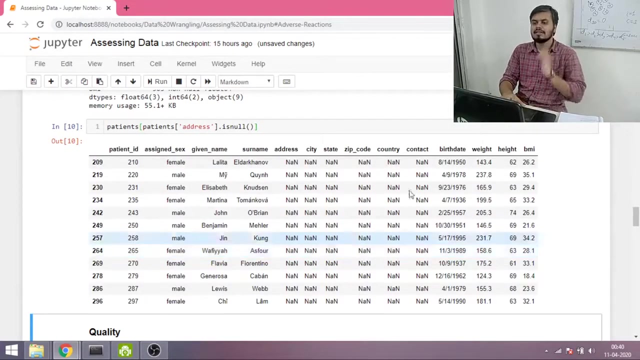 country and contact. in these 6 columns there are missing values, total 503 values in this code. so you can actually write this piece of code I will show you so you can write: patients address dot is null, right, or if I put this back in, 296. 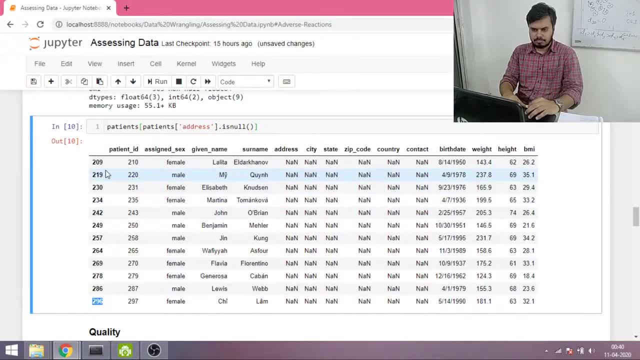 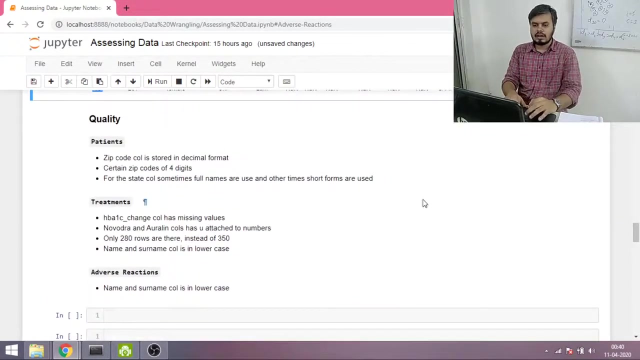 there are around 12-13 entries where address, city, state, zip code, country, contact. I don't have any contact record for these patients, so see again, we have to remove or fill it. that is our cleaning data, so I will go down and in the patients table. 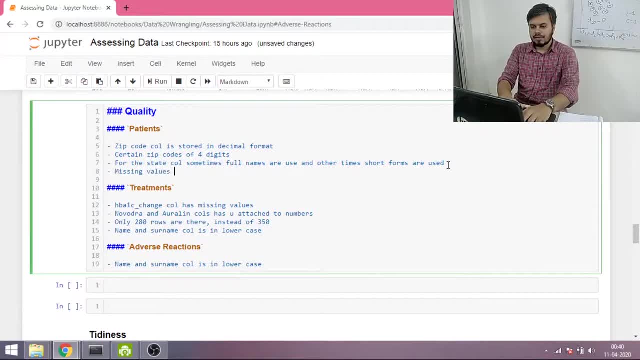 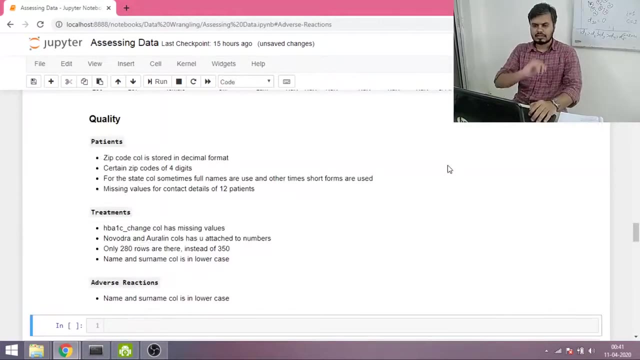 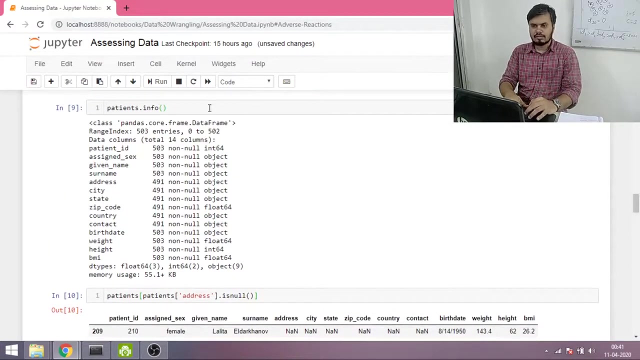 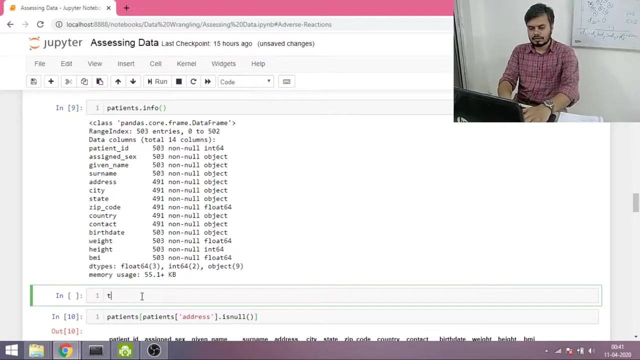 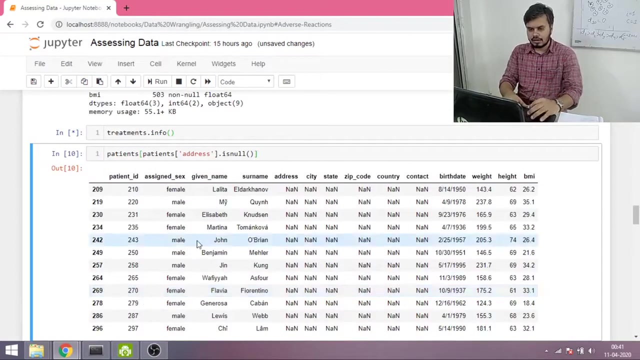 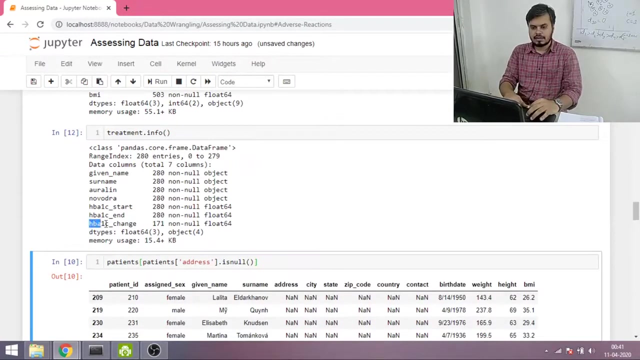 I will write missing values for contact details of 12 patients. so that is one thing that we got. similarly, if you, let's quickly check the missing values in the data frames. so we will run on treatments, we will run info and after running info on treatments, it is: 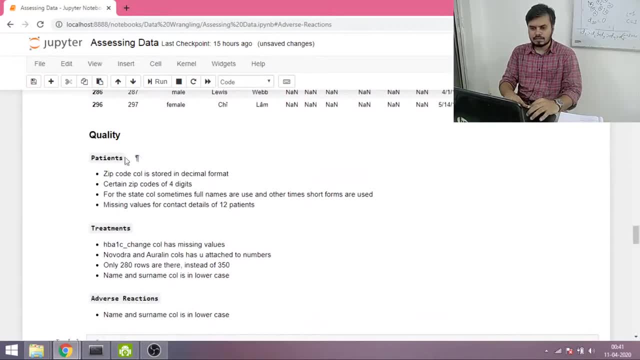 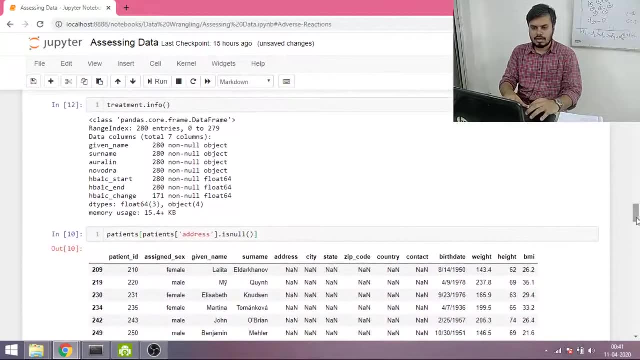 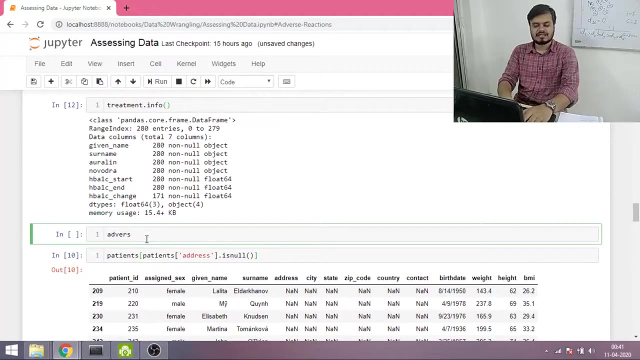 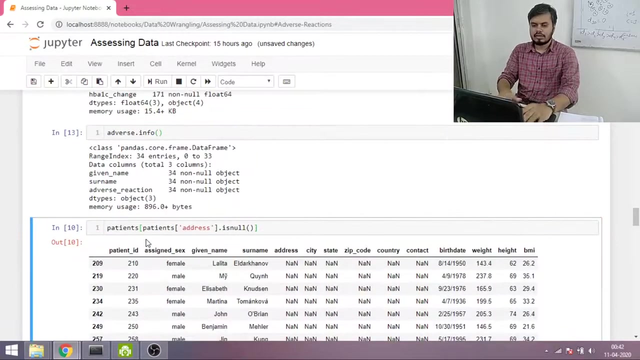 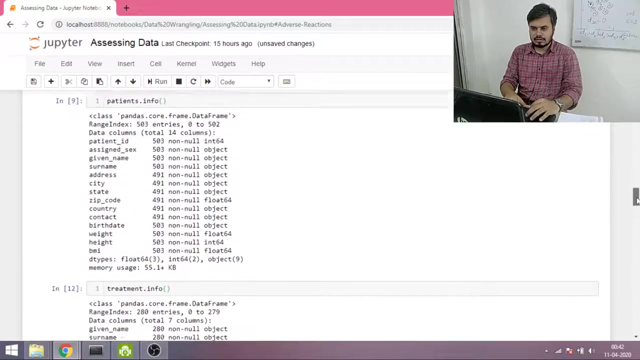 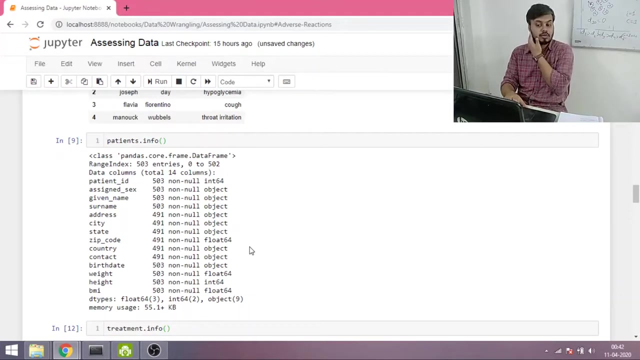 treatment. my bad. here we have written: hba1c change column has missing values. so there is no missing values here, last one that is adverse reaction, adverse dot info and we should get. so there are three missing values. next, what you should do is you should do. 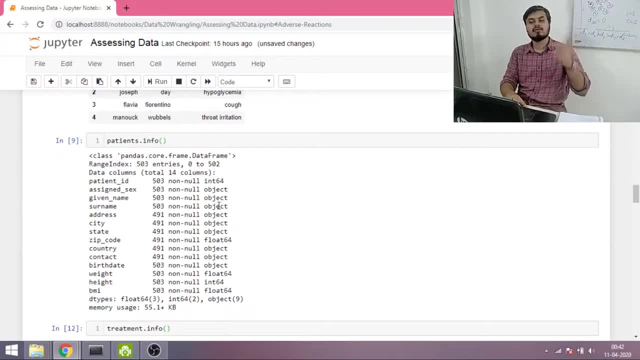 a assessment on the data type of columns, because there too many things are hidden. so what we will do is we will change it to category. so that is one thing. name is object. object is basically strings. ok, so that will work. surname is also fine. address is fine. 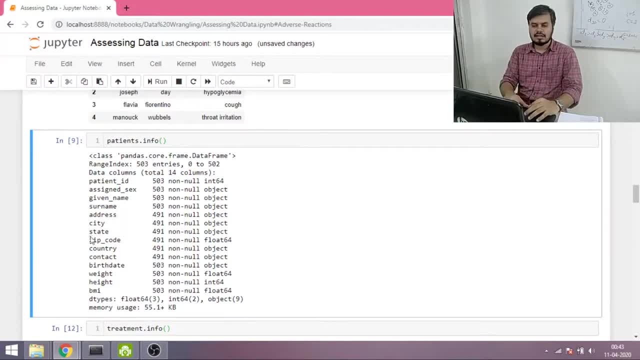 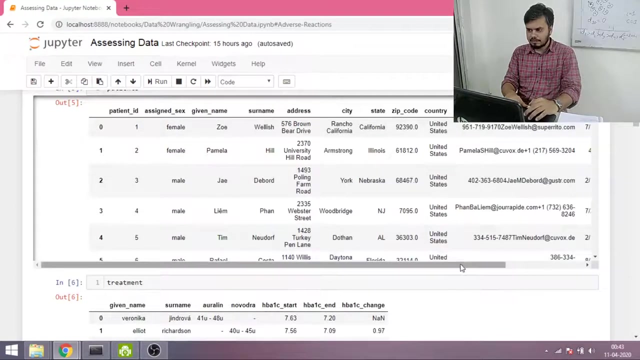 city. city is object. see, there will be many cities, so change it to category, not logical country. actually there is no benefit because all the patients are from US, so there will be no benefit. contact is object. fine, birth date is object, if I go to the data. so 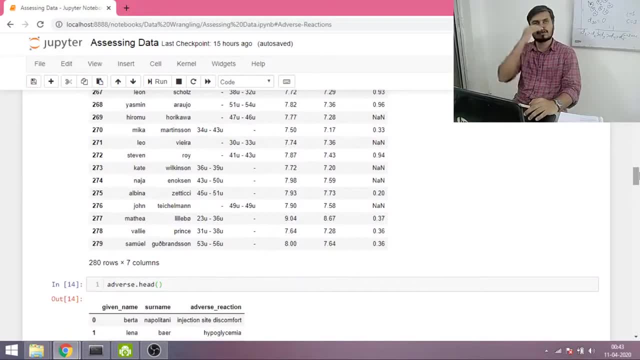 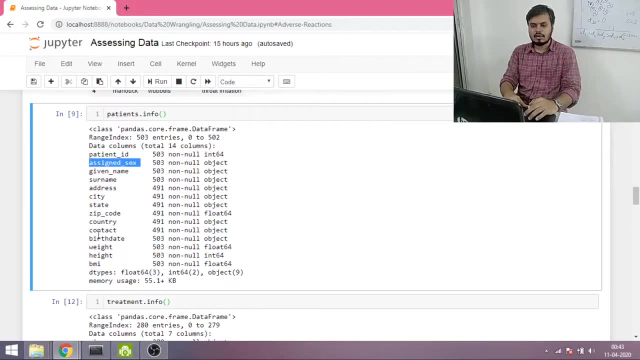 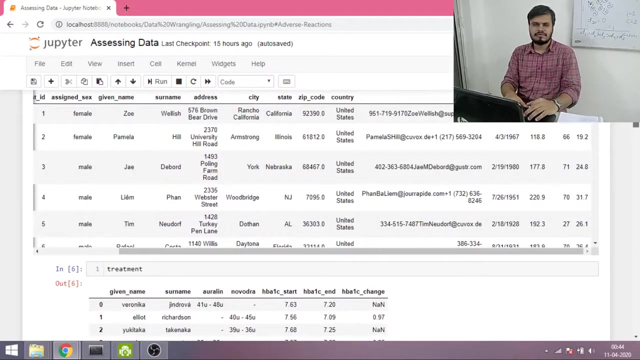 we will change it to date format, because sometimes you have to sort patients according to birth rate. so clearly, I have two columns at assign- sex and birth rate, which is not the right data. so fine, we don't have that data to represent, so it's okay. and 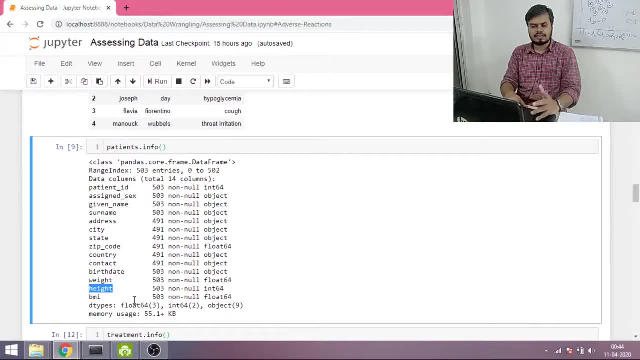 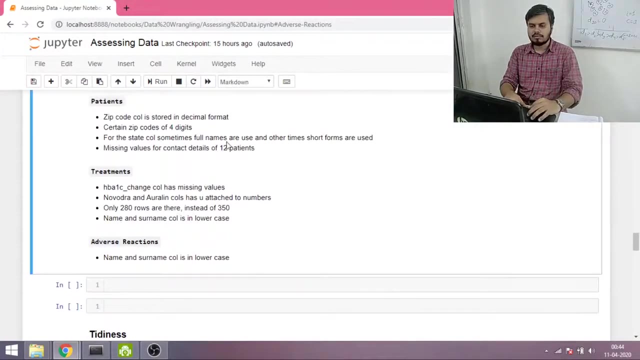 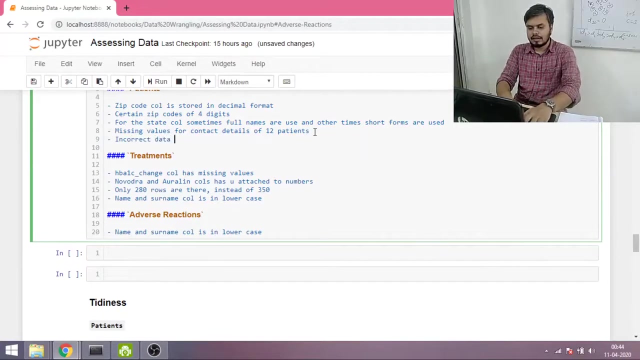 weight, sorry, height is in float, that is fine. BMI is in float. so after this assessment, we understand that we have to change the data type of assigned sex column and same with incorrect data types, for first one was assigned sex, assigned sex and second one was, I guess. 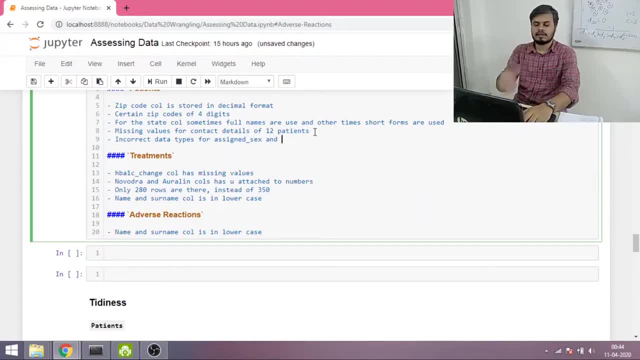 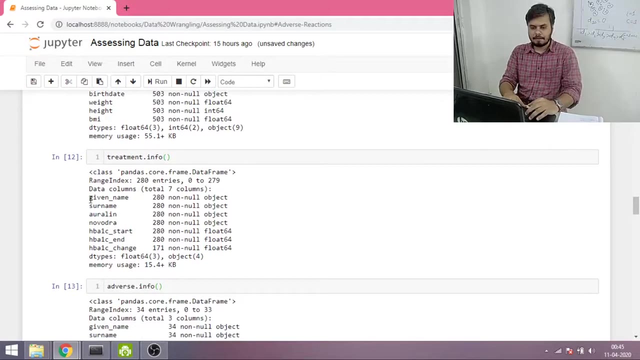 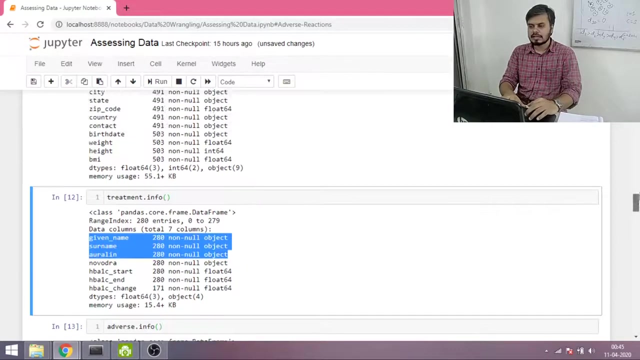 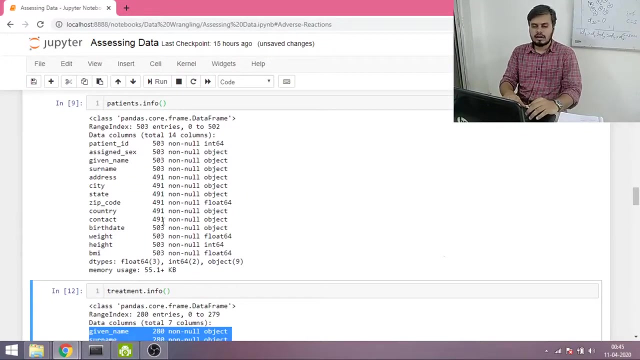 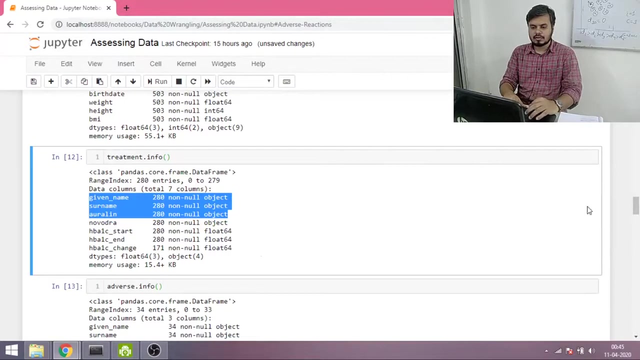 birthday birth date. birth date columns. okay, this is done. now we will do same assessment on the treatment. so let's talk about treatments. in treatments, given name should be object surname. object: oralin and novotra. this is numerical data and stored in object. so we have. 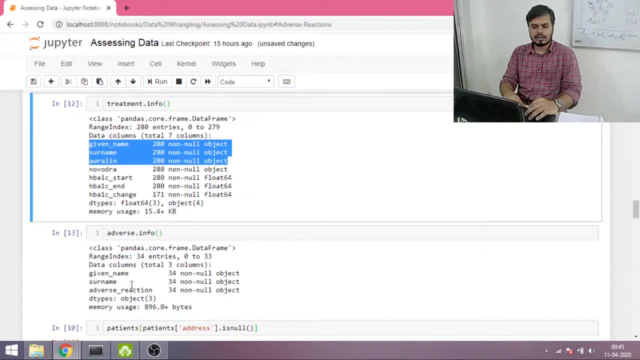 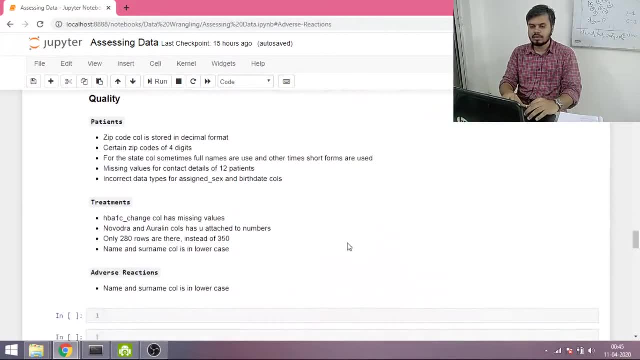 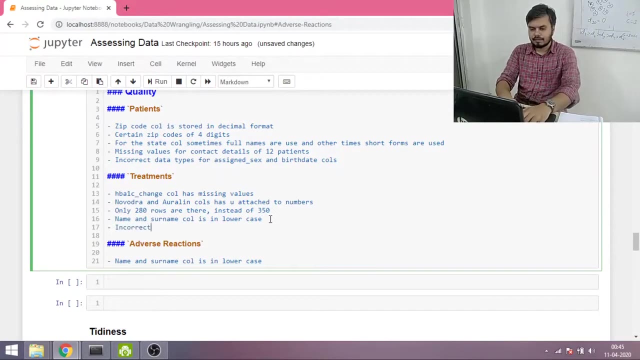 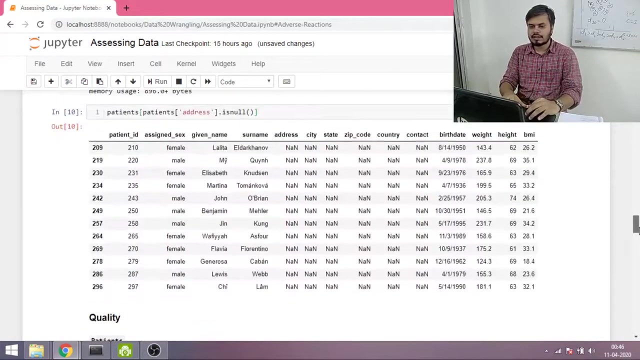 to change this and after H1 type. okay, so we have in treatments table one quality issue, that is, the incorrect data type for oralin and novotra columns. okay, this is done. next is next. what we will do is we will try some other functions like: 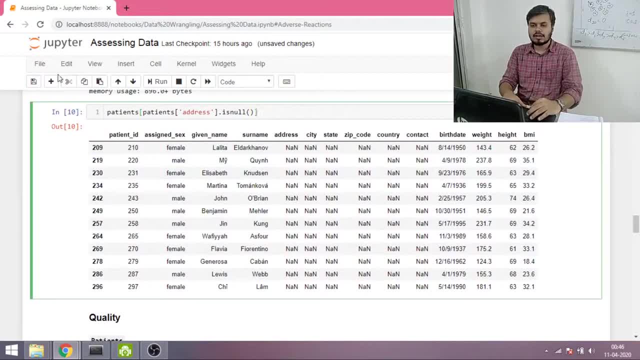 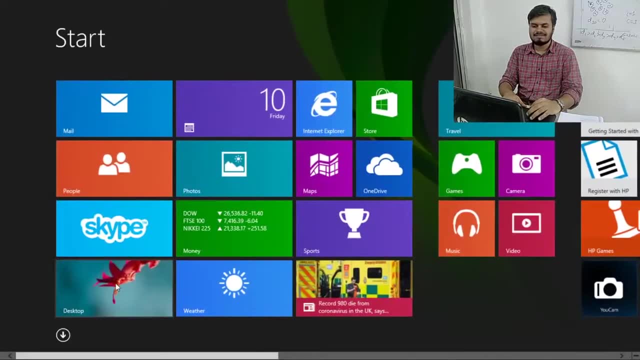 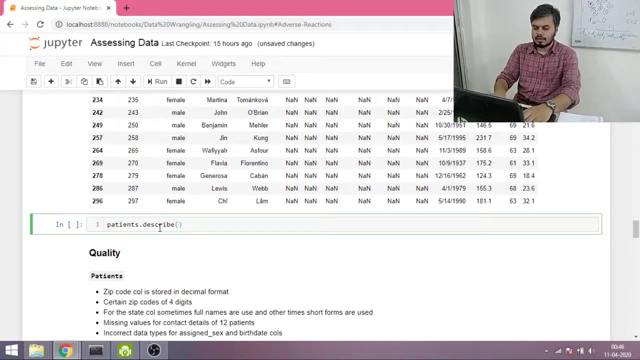 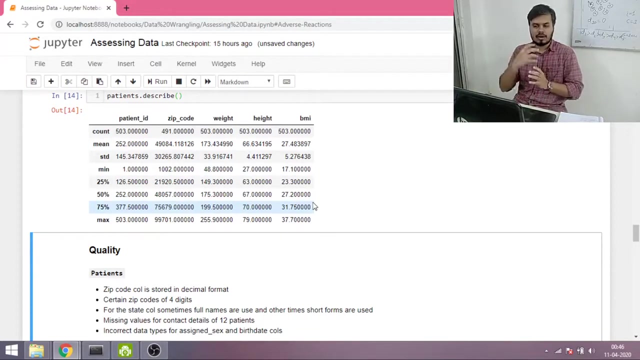 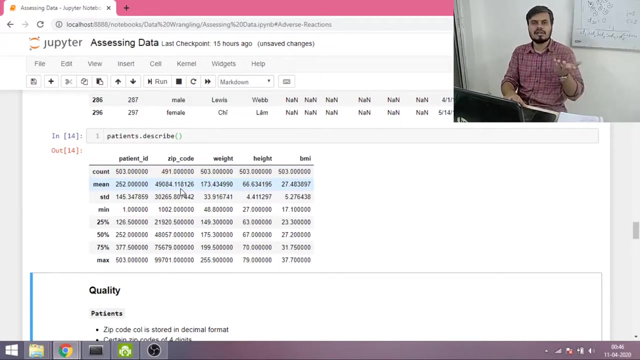 one function is describe. I guess you know it is applied on numerical columns. okay, so let's apply describe on patients, let's see what result we get. sorry, so if you can see, count mean standard deviation, min and all quantiles, and we have five numerical columns: patient. 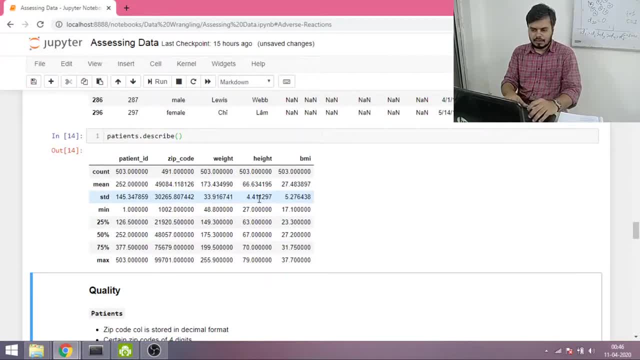 id nothing in this is nothing there. so there is weight, height. this is an issue. I will show you. we have height in inches and, if you notice so, minimum value of height is 27 inches, 27 inches that is. that is very small, like 27 inches. 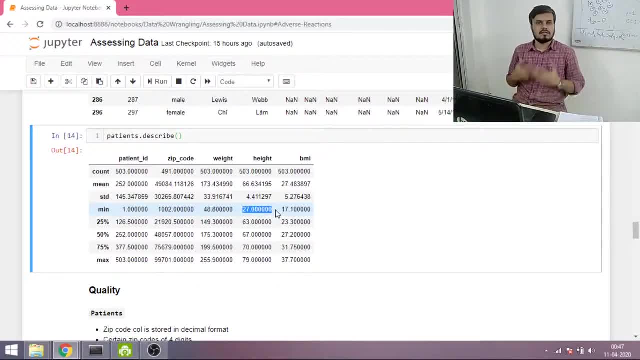 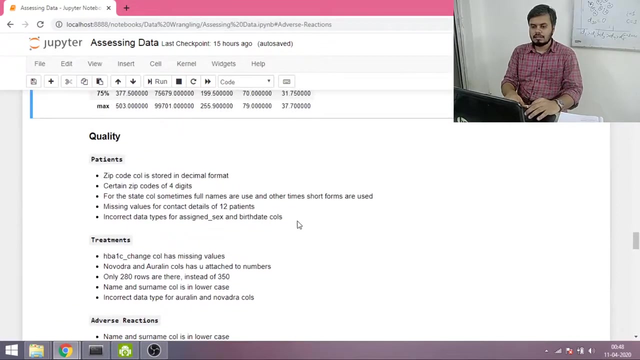 human being, that is. that is not possible. this is incorrect. data 27 should not be there. we have to pay attention to this, because our mathematics calculations can be wrong. similarly, we are taking weight in pounds, and there is this guy whose weight is 27 inches, so 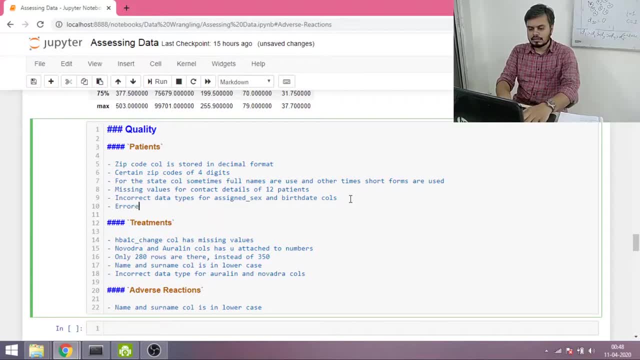 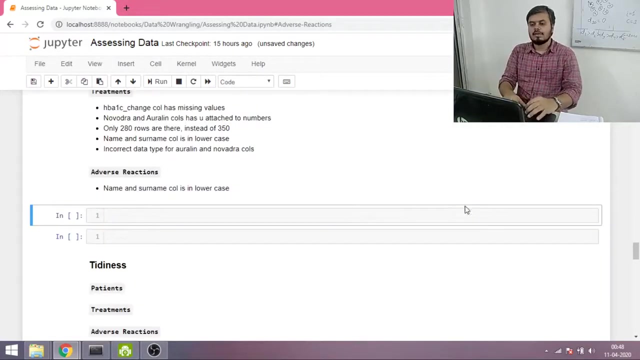 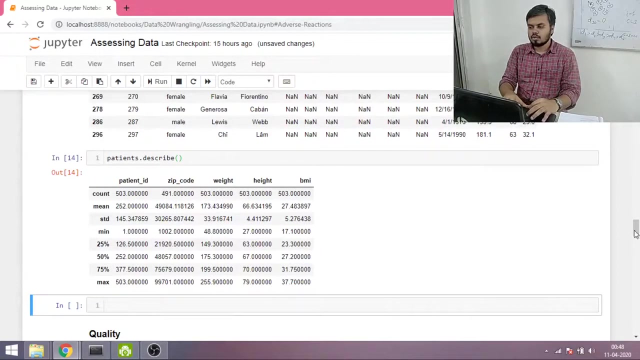 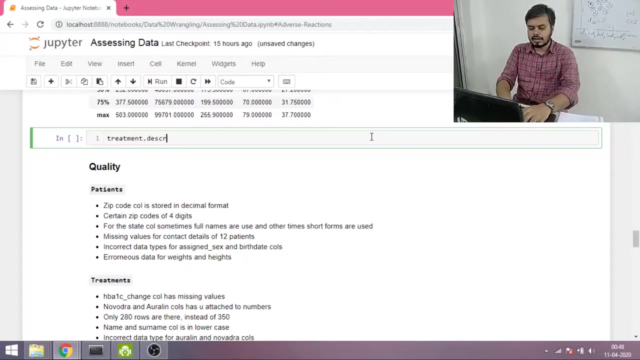 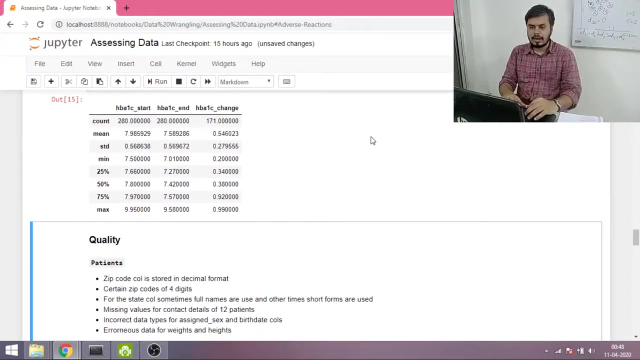 we will write in patience that error in is data for weights and heights. ok, this is done. next we will write in patience that next we will put describe on treatments. so we will write treatments, treatment, actually treatment, dot. describe. and if we run this code, yeah, so here. there is a major problem. I noticed that HBA1C change. so minimum is 0.2, 25% is 0.34, 50% is 0.38, but 75% is 0.92. so sharp jump between 25%. 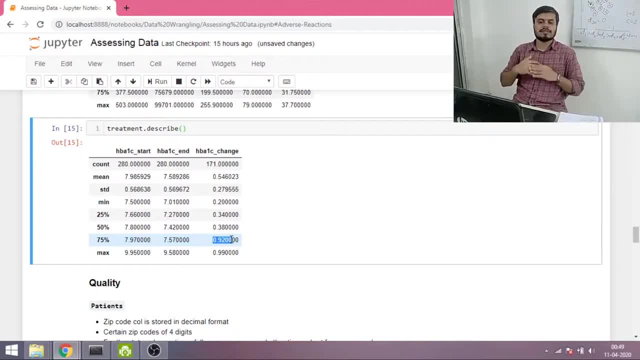 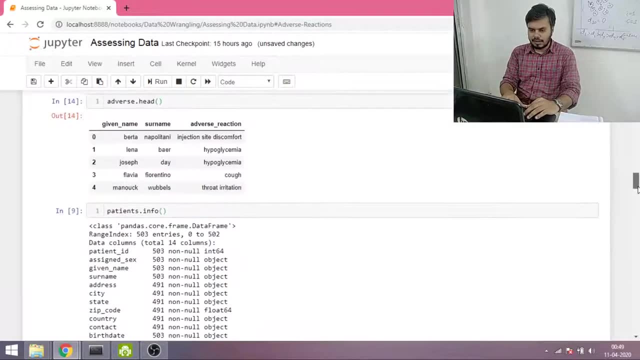 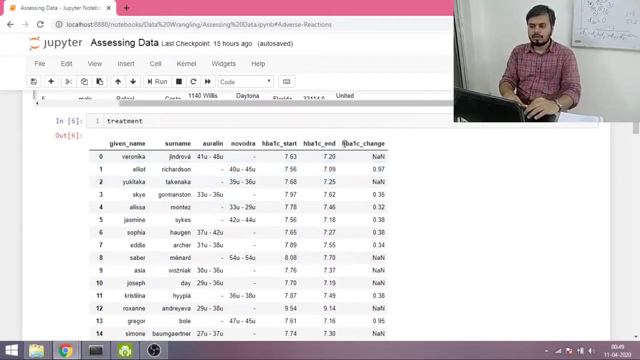 value. sorry, 50% value and 75% value. ok, and when I backtracked, I will show you what is the problem like. see here this data. I said this column comes after subtracting these two columns, right? so see here: 7.56 and 7.09. 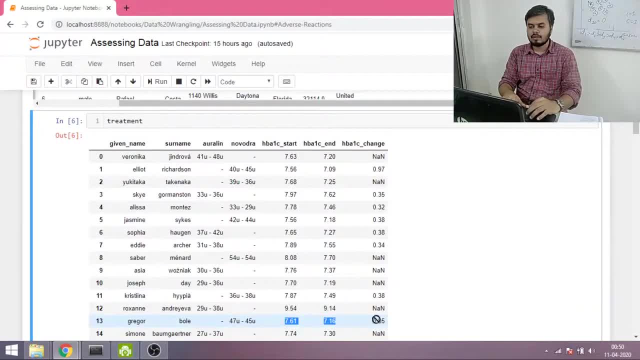 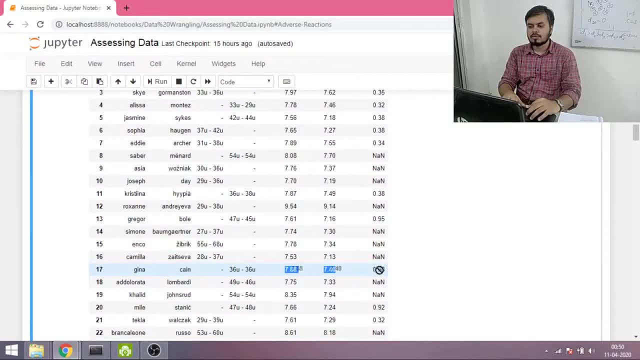 should be 0.95, ok, 0.95, and wherever you see 9, you will notice: here 0.48, here it is 0.98. so somehow, 9, 4 is 9, 4 is 9. so now, whatever reason is, 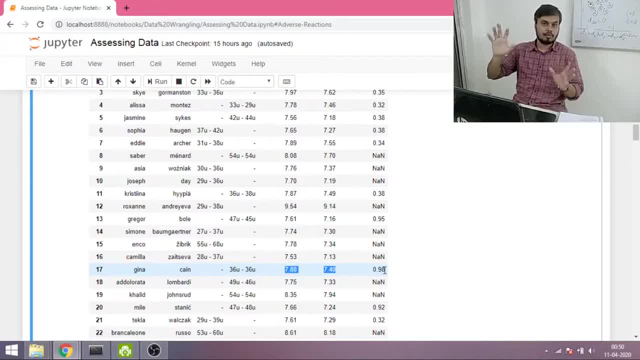 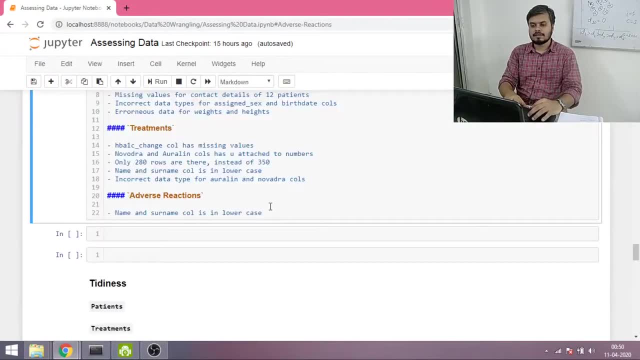 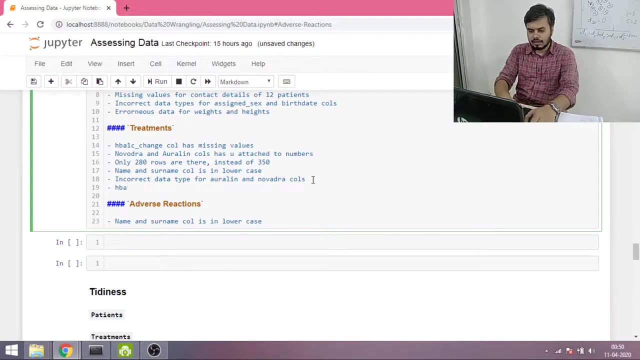 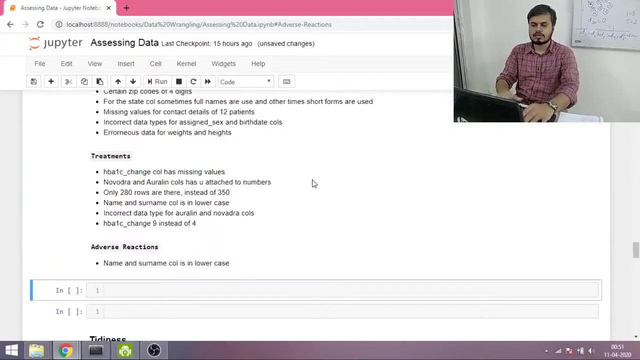 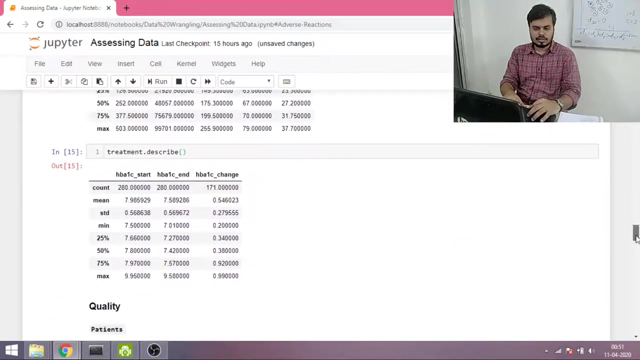 there the handwriting is 4- 9. that could be one possible reason, but whatever is here, we have to do a major change in our treatments table. in the next. we have to rectify this, ok. next, if we have used describe, so next we will use a very 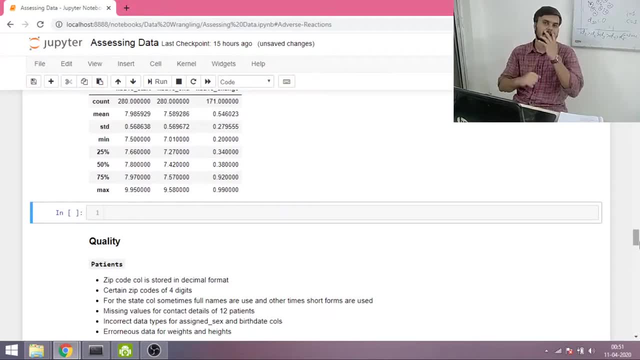 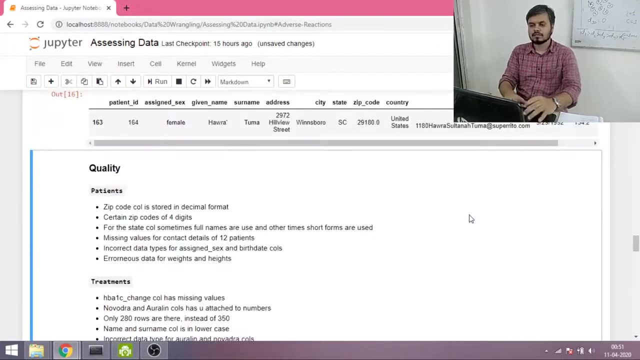 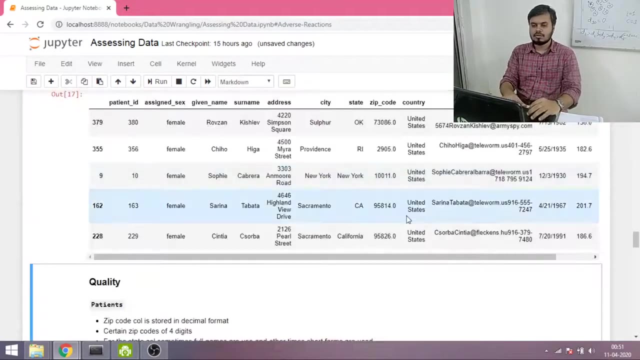 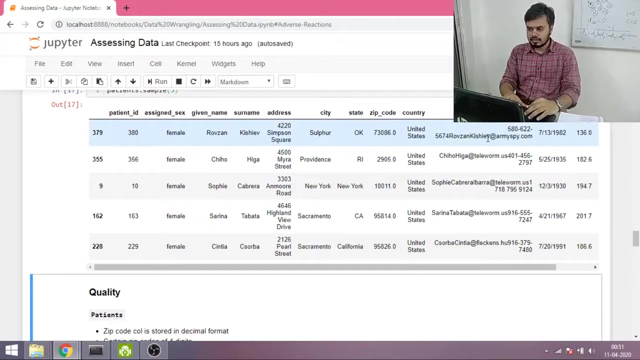 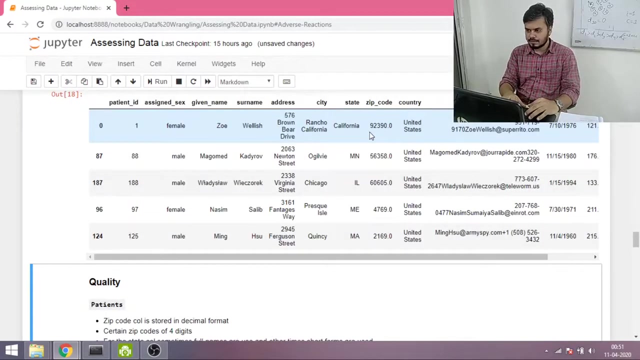 good function called sample. sample randomly gives you a row from your data frame. so if you put 5 in it, then you will get randomly selected 5 rows. ok here. one thing to notice is that is actually. I noticed this earlier. let's run it again so that. 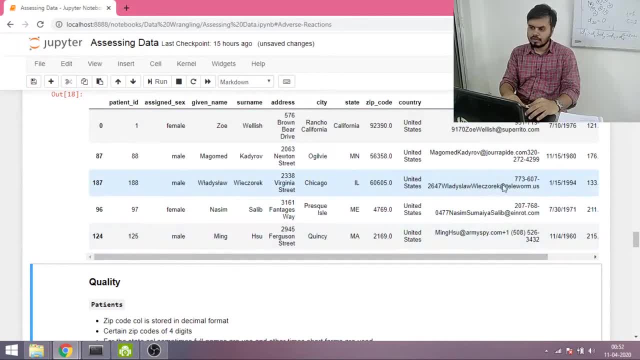 there are more. you will notice that phone numbers are stored inconsistently. ok, so 951719 and 9170, 320, 272, 4299, 773, so basically 3, 3 and 4, but suddenly there are certain phone numbers which are looking like: 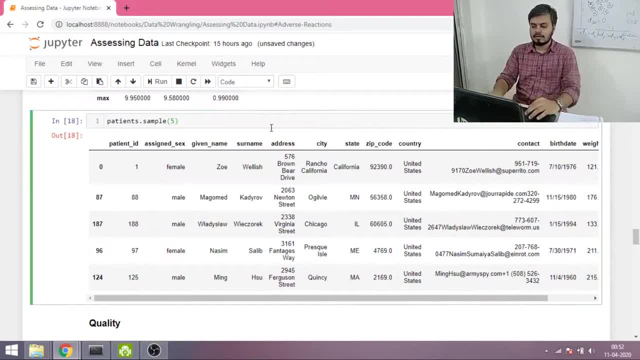 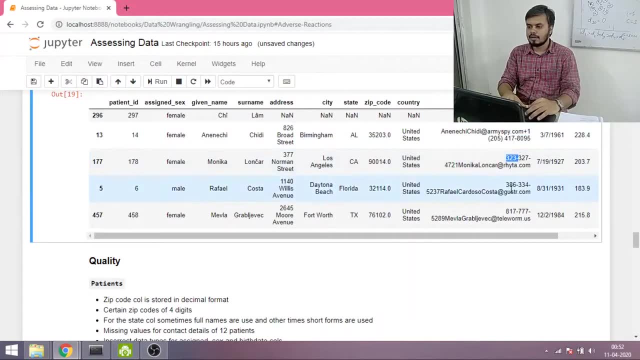 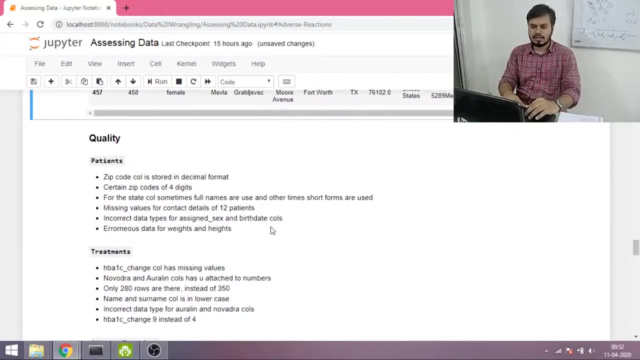 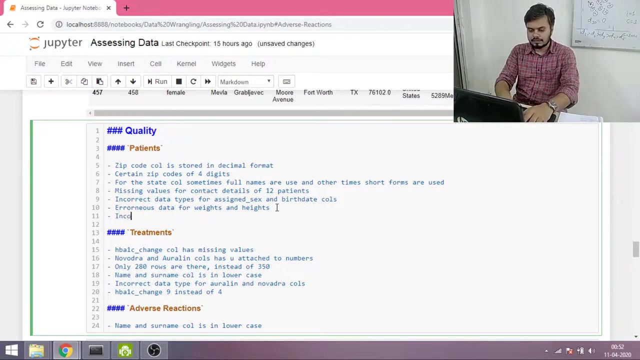 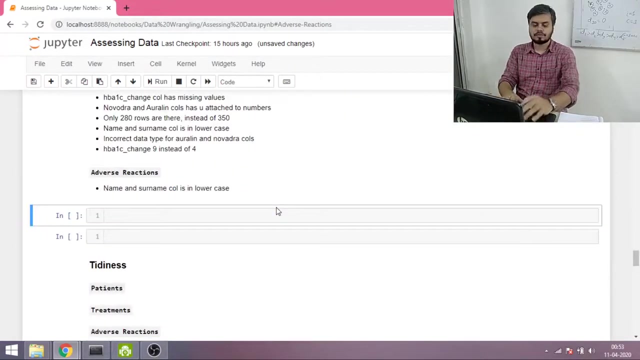 this, so inconsistently phone numbers are stored, which is obviously not good. I will show you some more examples, like here: 205 brackets here, normal. here, normal here, normal, ok, so inconsistent way of storing for phone numbers in contact column. ok, this is one more issue. the next: 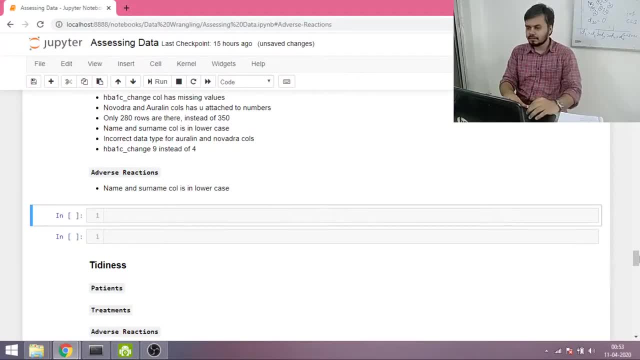 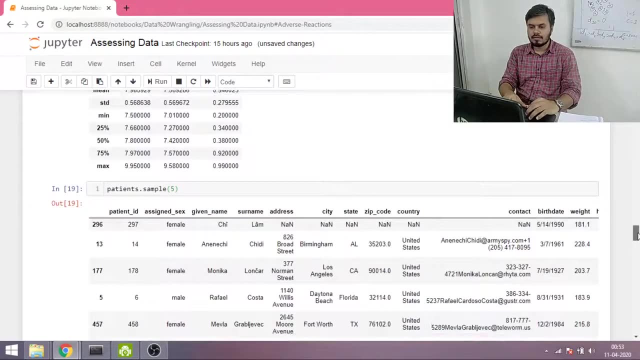 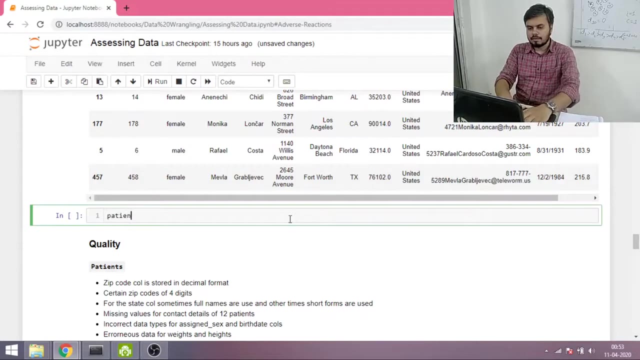 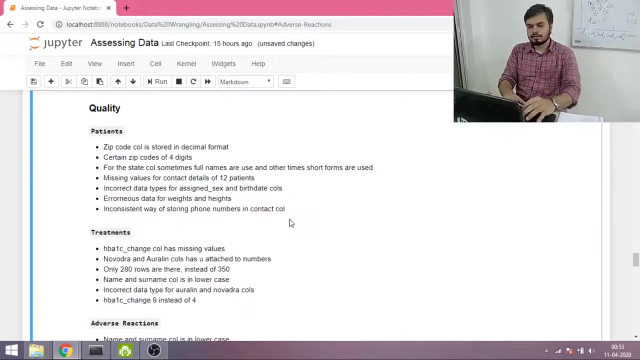 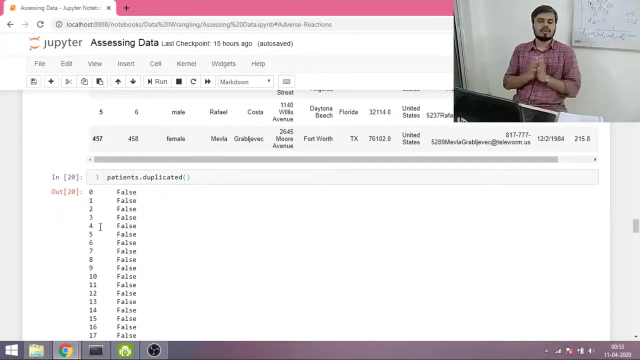 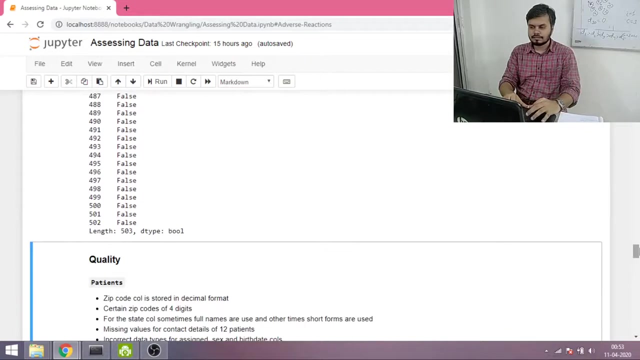 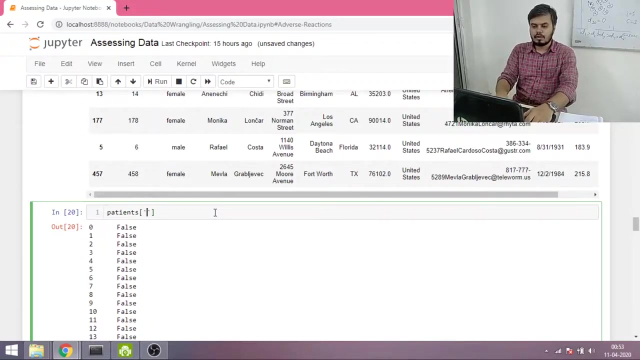 issue is duplicate data. so I have got this issue in patients column. I will show you, and you should check, if you put duplicate on your data frame. what this will do is this will tell you that your whole row is not duplicated. ok, so at this point all. 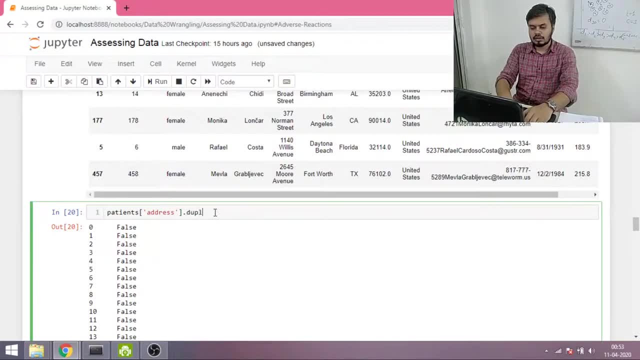 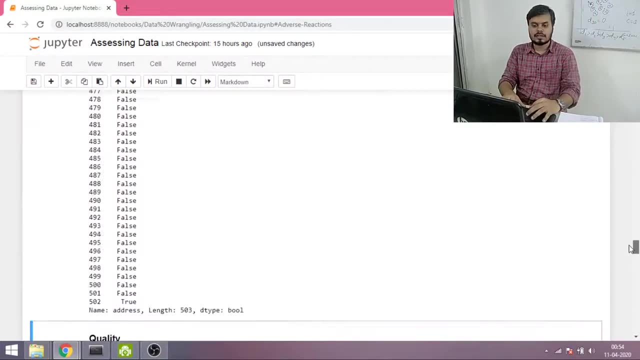 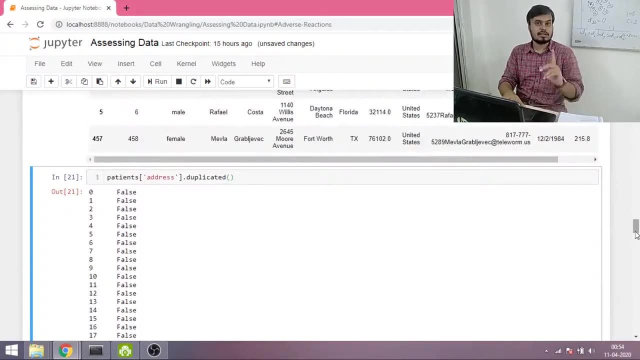 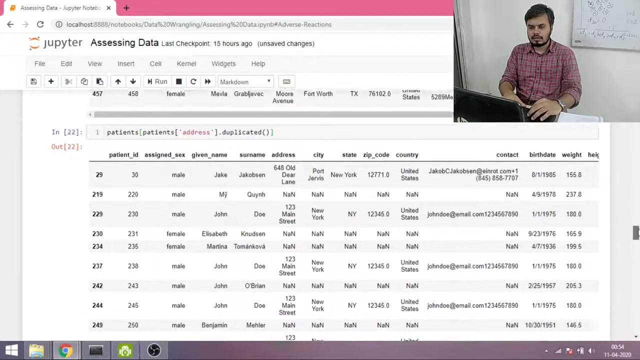 this address dot duplicated: ok, here I got some true values. means some patients were like this: see here: last is true. so basically some patients were like this whose address was repeating: ok, it means it should be same patients. but when I backtrack, means this: this: this is the detail. 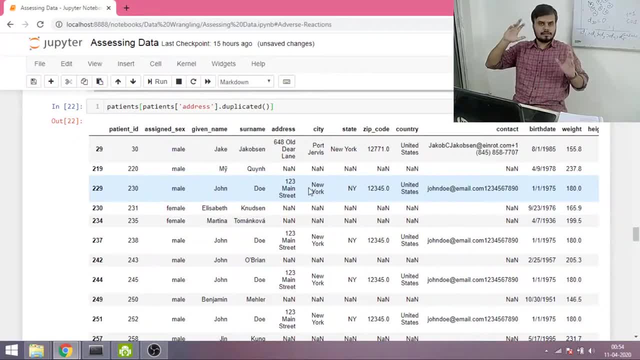 of all these patients whose address is duplicated twice. ok, minimum twice. so you will notice that, like this guy, his first time this address has come, this is not so problematic. this is repeated value. one, two, three main street. one, two, three main street, and every time patient's name is: 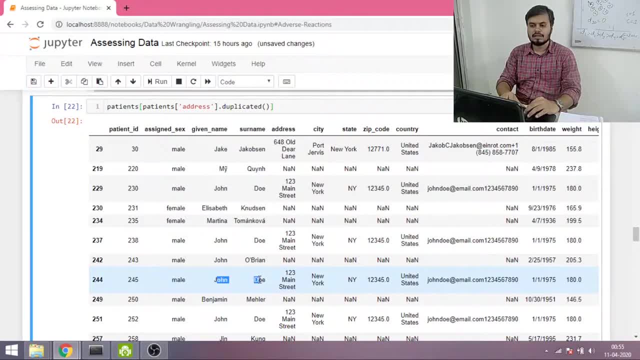 John Doe. now, if you have done web development, you would know it's basically a place holder. John Doe is basically a place holder. whenever you design any design, you write John Doe, it's a place holder. so in this data somehow there are five or six place holders. 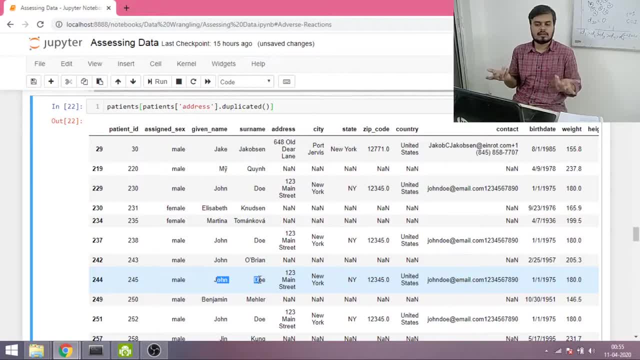 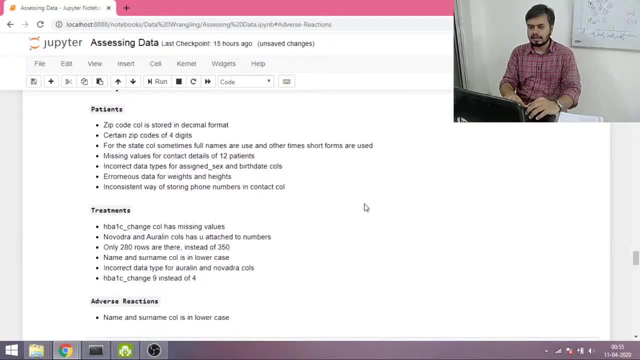 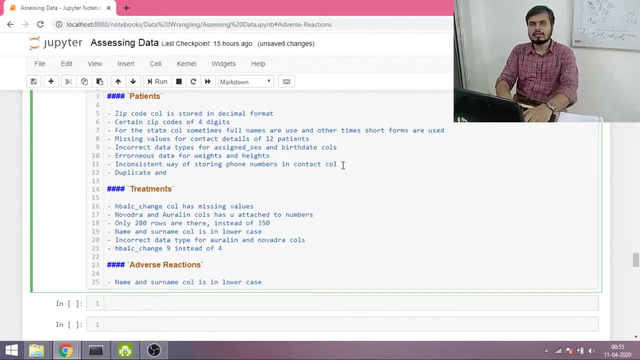 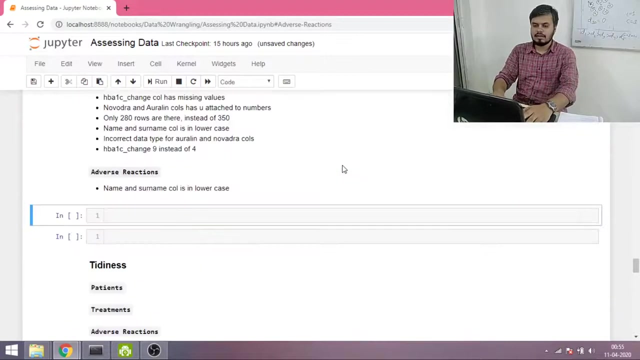 for patients. ok, so obviously this data is useless and it has to be eliminated. ok, so we will write duplicate data duplicate. and what should we write? this is not useful, not useful, let's call it not useful. data in data set. this has to be removed, ok, ok. 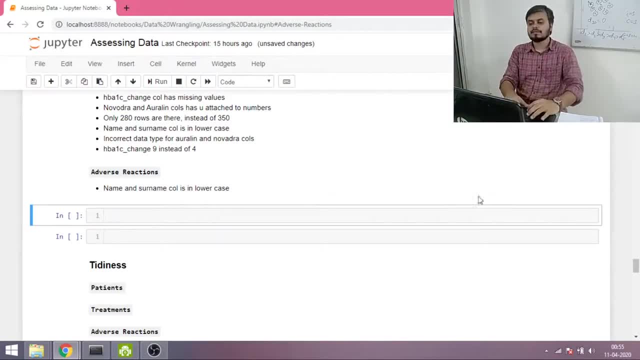 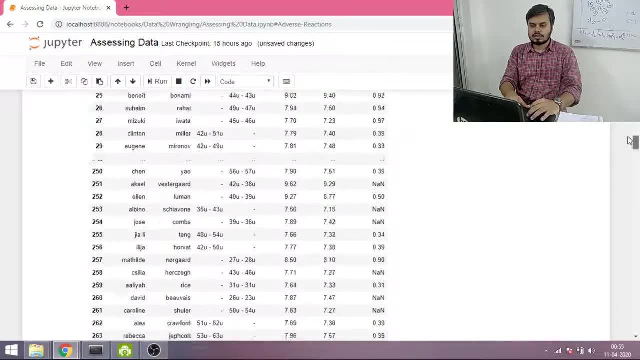 the last thing which we will know from the programmatic assessment, and you might have seen this before: if you go to this treatments column then you will notice that in the treatments column some passengers- I am really sorry- some patients we gave Auralin and some patients. 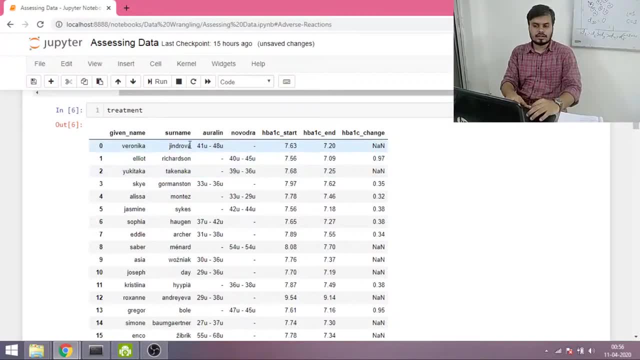 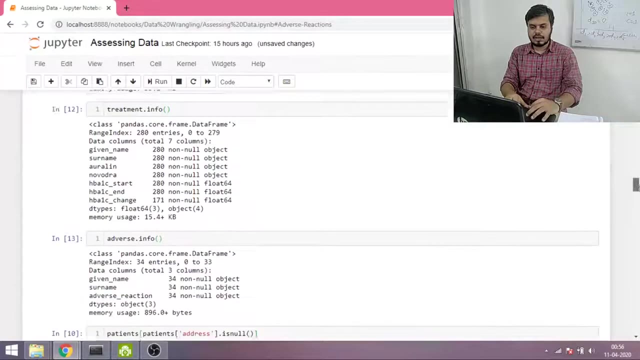 we gave Novadera. so the one who was given Novodera, his Auralin has to be blank, and the one who was given Auralin, his Novodera has to be blank. ok, but if you notice when we run info then it shows. I will show you. 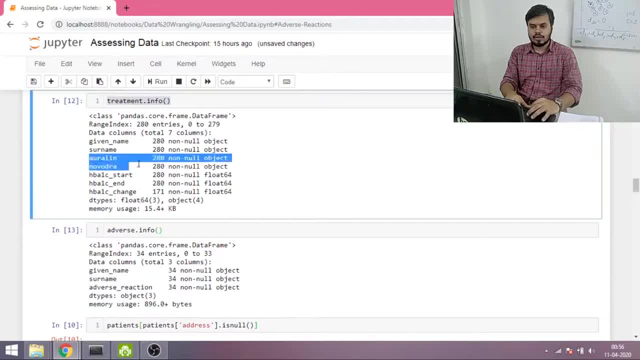 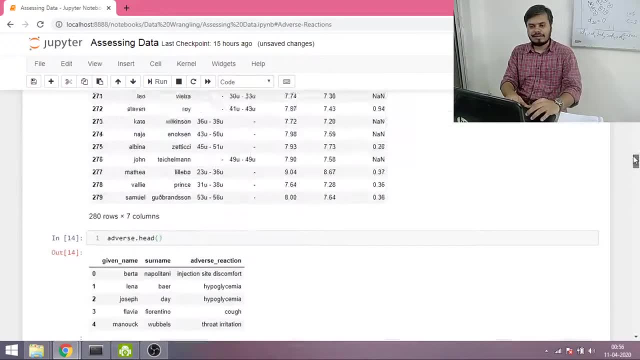 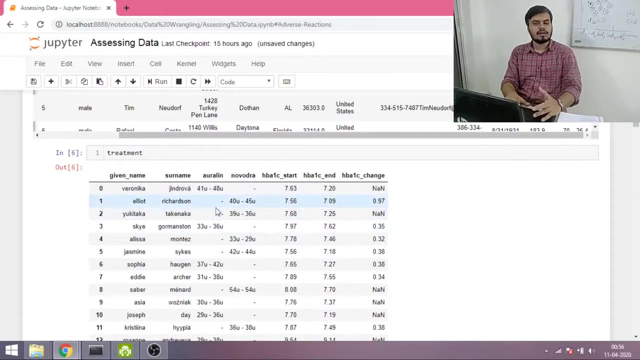 that when we run info on the treatments, then our Auralin is also showing 280 and Novodera is also showing 280. it is because there are no null values. these values, they should have been null, but these values are not null. these values are not null. 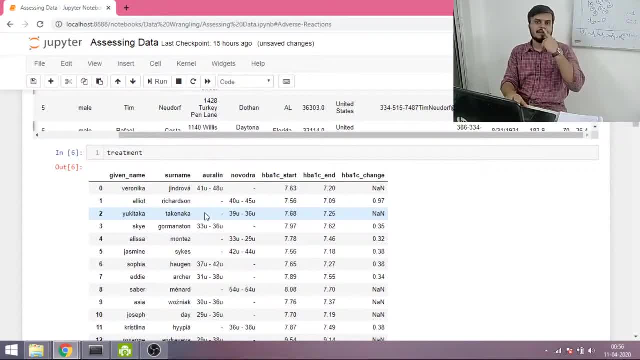 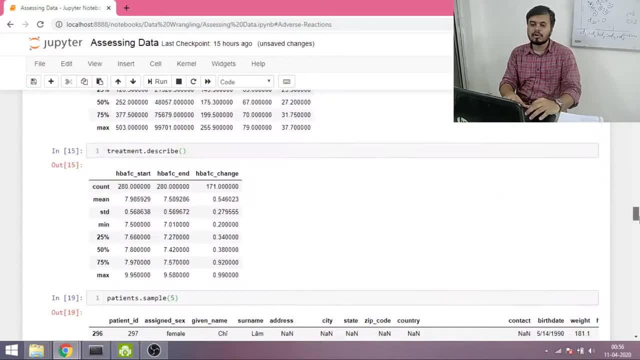 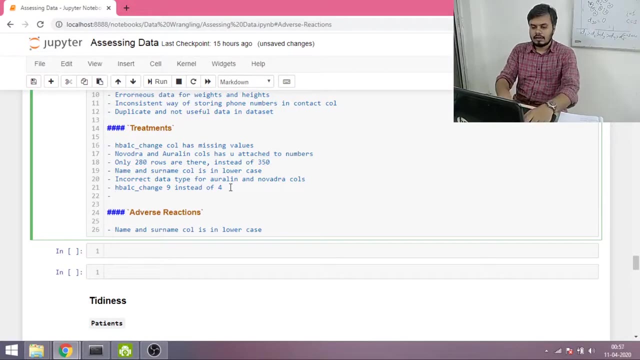 instead we have put dash there. ok, and obviously putting dash is bad, null is better. null is in our control, right, so we will document this as well and we will write in the treatments table that use of dashes instead of NaN in Auralin and Novodera. 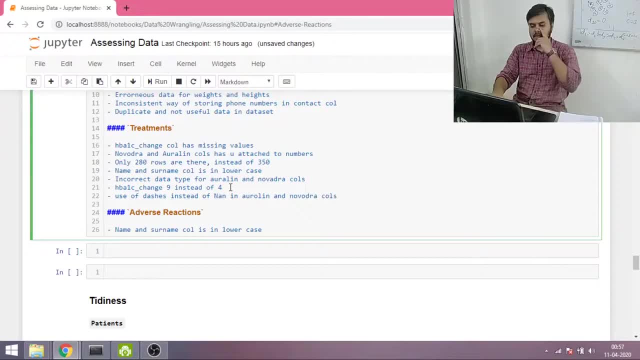 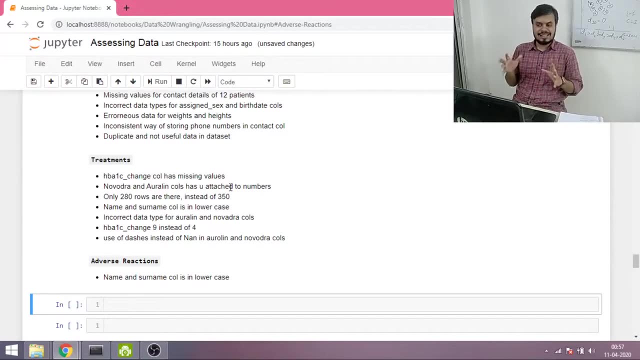 columns. ok, so, guys, this was our programmatic assessment, or our programmatic assessment, and next we will talk about the quality of the data. we will talk about the untidy data. ok, we have taken out the quality data. now we will focus on the tidiness issues. 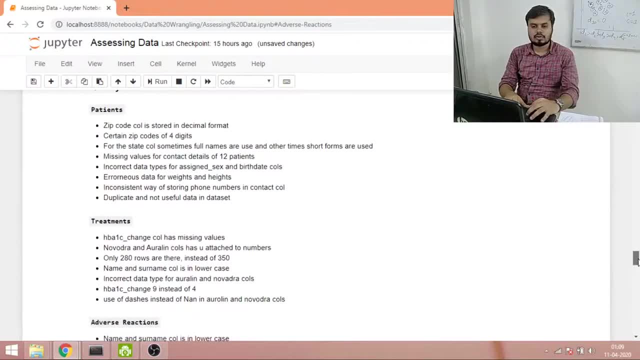 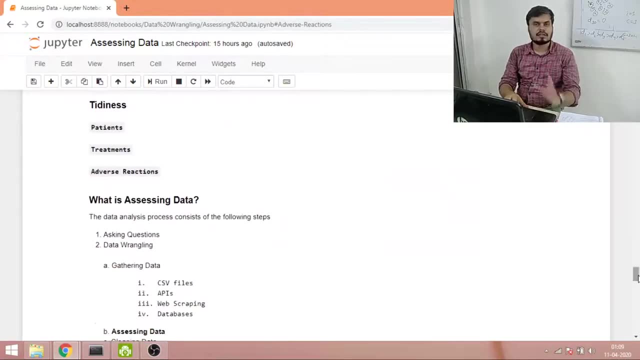 ok, guys. so now we are done with the quality issues in our data. there are a lot, see, we have to correct a lot of things. now let's move on to tidiness issues. ok, structural problems. so, as I have seen, there are 3 problems in this data. 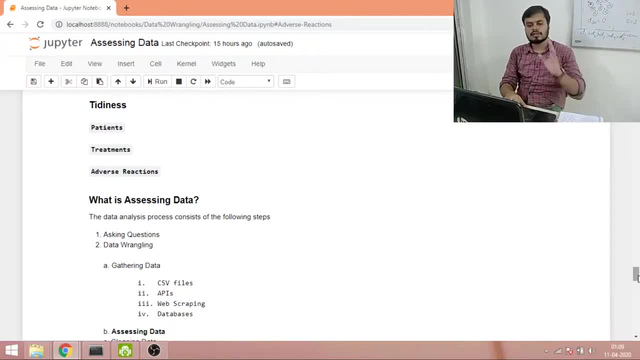 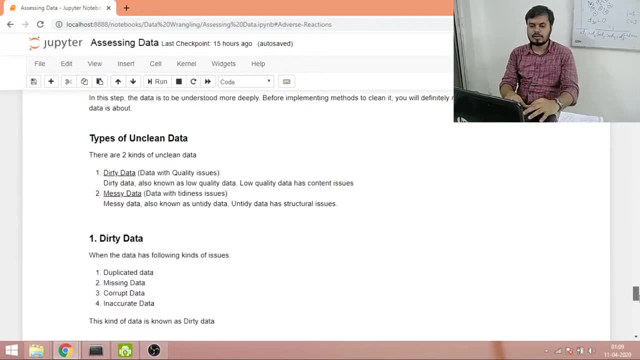 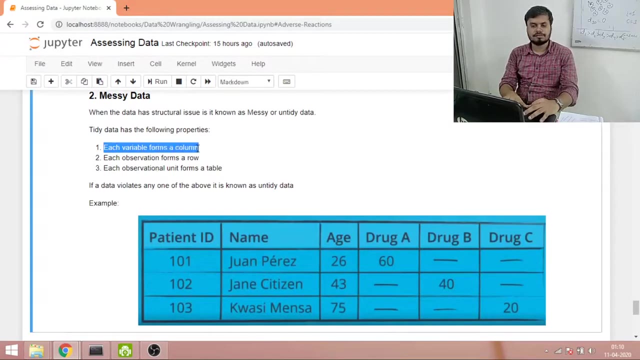 I will show you one by one. there is one problem in all 3 tables: ok, patience, treatment, adverse reaction. there is one problem in all 3. I will show you. the first problem is with the untidy data. each variable forms a column. each independent variable forms a. 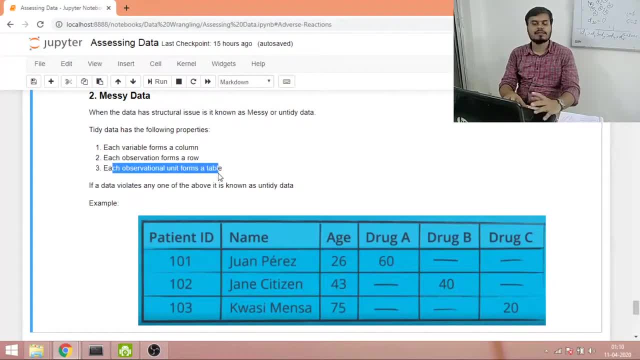 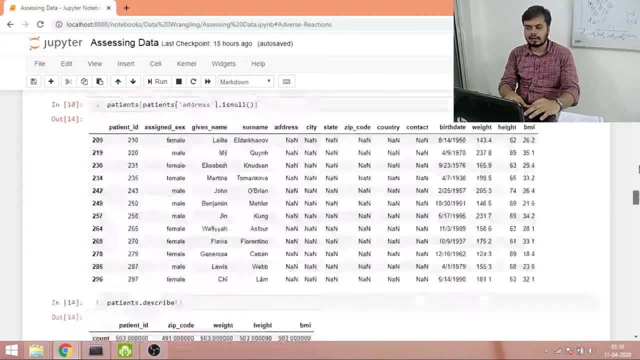 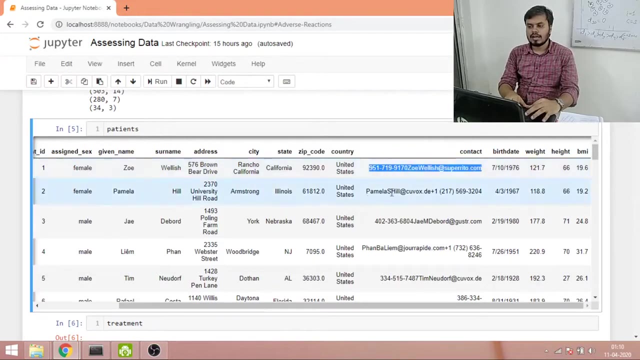 column, each observation forms a row and each observational unit forms a table. these are the 3 rules. ok, so the first problem is that we are putting 2 pieces of information in one column. we are putting phone number, we are putting email, so this is the first. 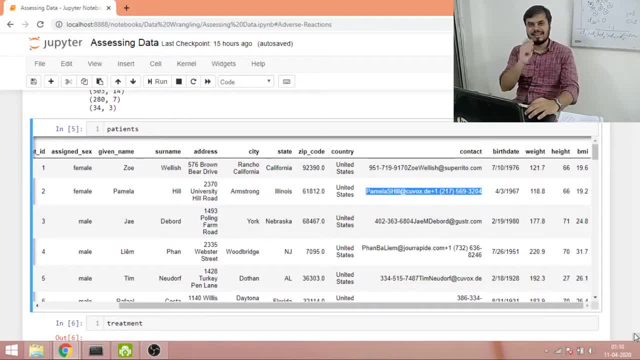 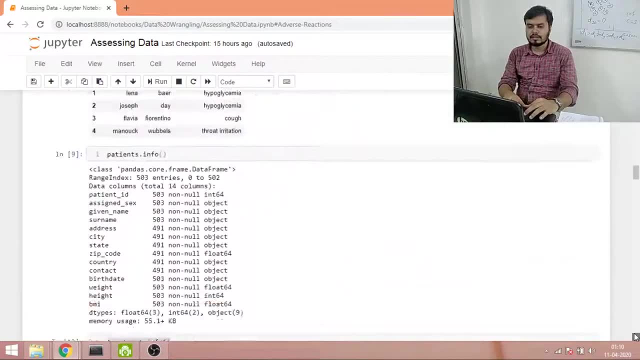 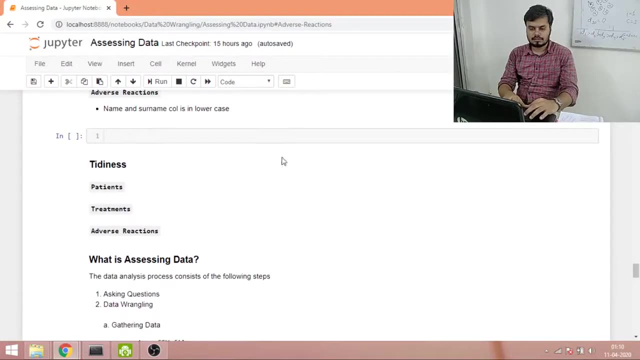 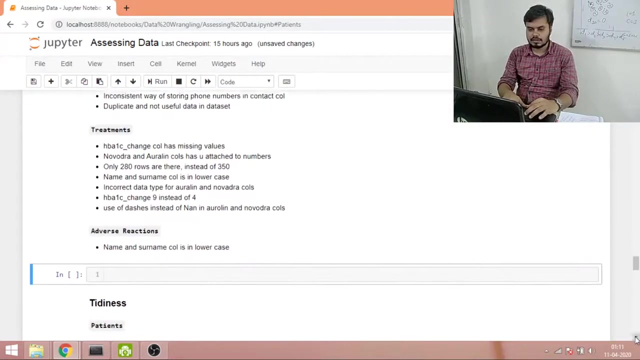 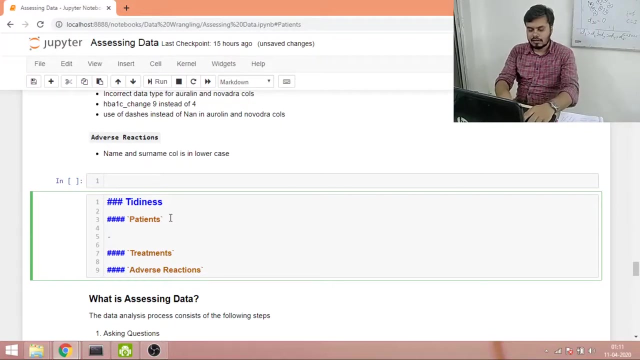 problem. this is untidy. here each variable is not forming a single column, so we will rectify that. before that, we will document it. so let's go to this place. yeah, patience, not this one inside. patience will document it. we will write remove or we can write. 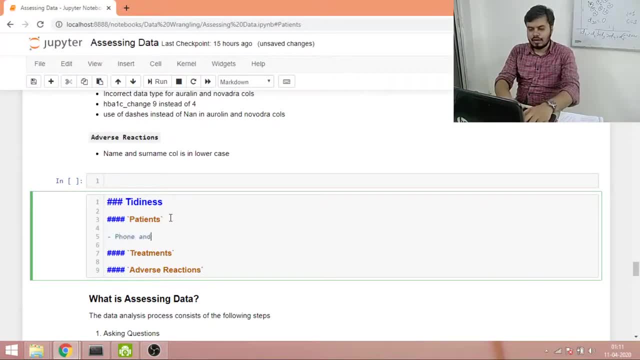 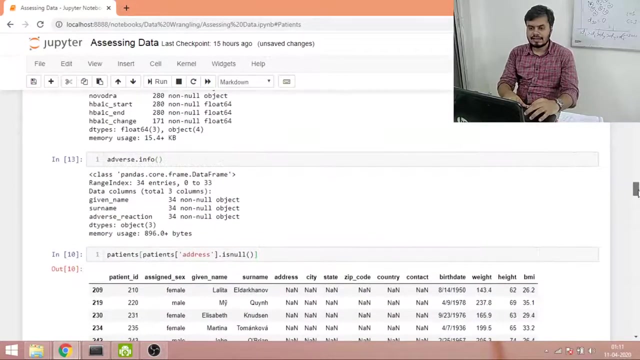 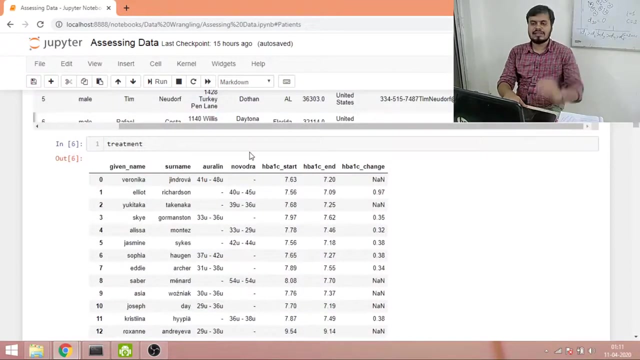 that phone and email together in one column, that is one column, the contact column. ok, so this is the first issue. the second issue, again a very logical issue, is present in this table treatment table. I will show you. yeah, so if you notice here whoever created this data? 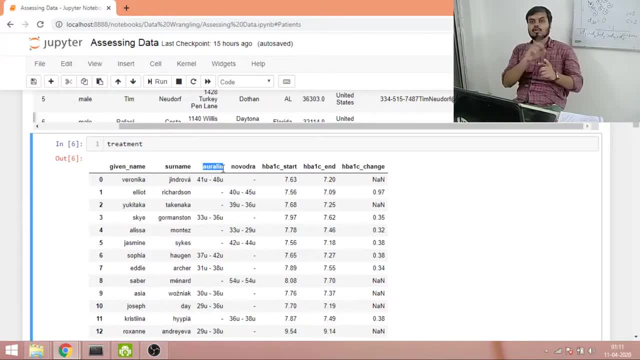 stored things in a column. so how this table was organized, it made one column for auralin and one for Novotra, right by the rule. if you think about it, here are three pieces of information hidden. first piece of information is: how much lower dose? second piece of: 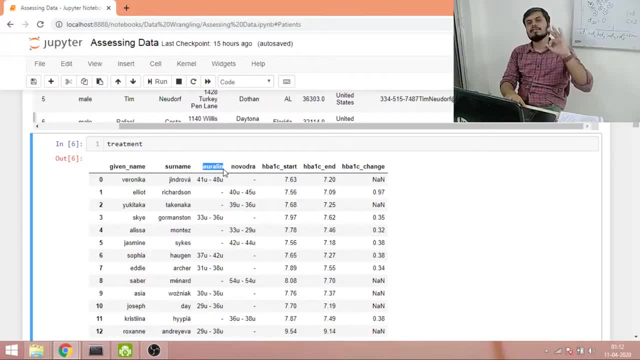 information is how much higher dose, and third piece of information is which medicine. this is why this is not correct. we should have made three columns: first, lower dose. second, upper dose. third, treatment type: auralin and Novotra. ok, I hope you understand. so we will. 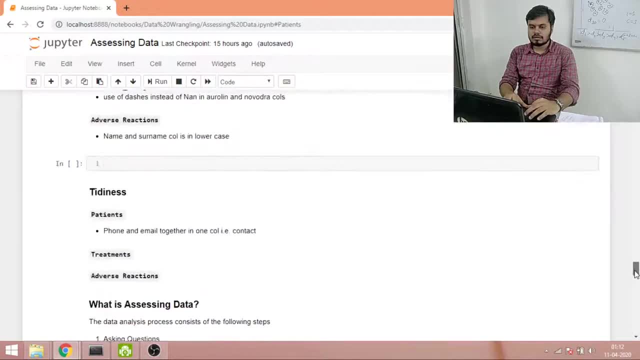 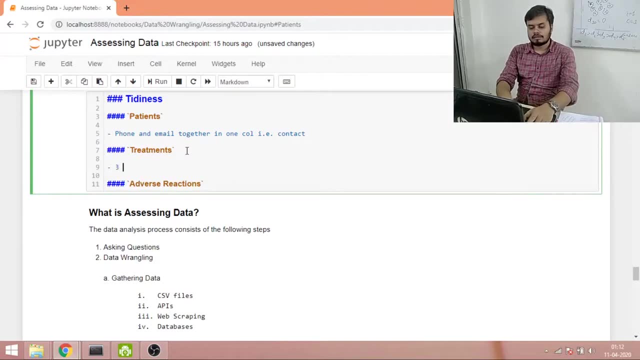 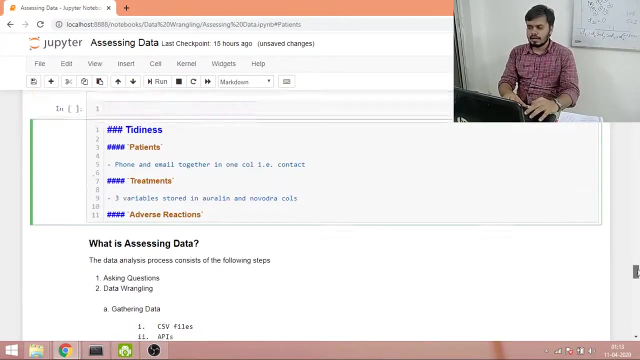 document this. so we will write inside treatments table. we will write three variables, variables stored in auralin and Novotra columns. ok, this is the second problem. structural third problem: if you notice carefully, this table, which is not noticed constantly, is the adverse table. basically what? 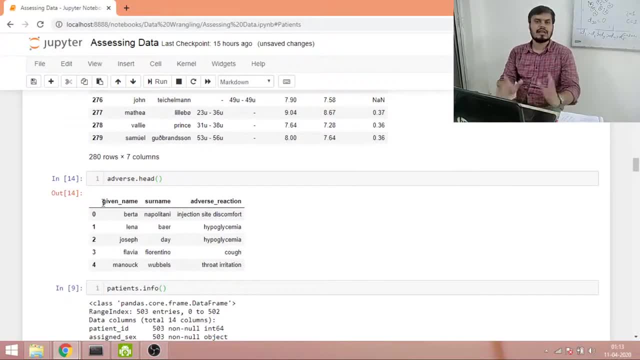 happens in this table is: we gave medicine to 280 patients and in this table we noted down the name of those patients with whom there was some adverse reaction of the medicine. ok, now this total is 34 patients out of 280 patients, so basically these are the same patients. 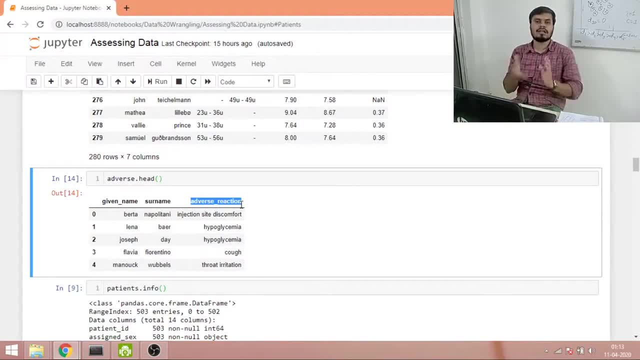 right now, just to store this information that they had adverse reaction. I made a separate table. this is not logical. this separate table is: I will take this adverse reaction column and put it in the treatments table. those patients who had reaction will write the type of reaction. those who did not. 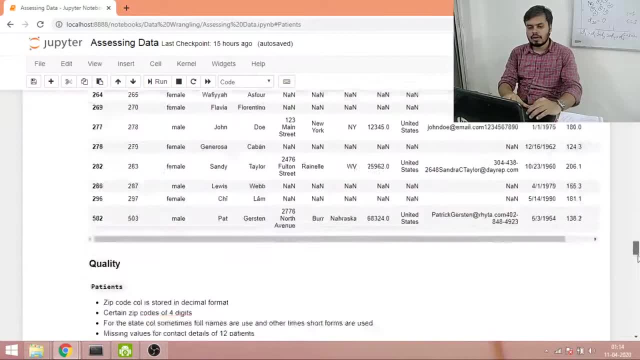 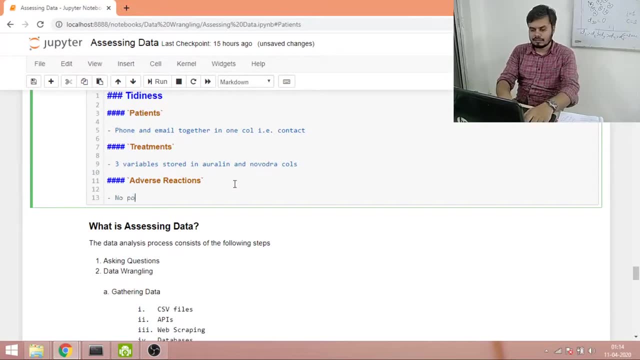 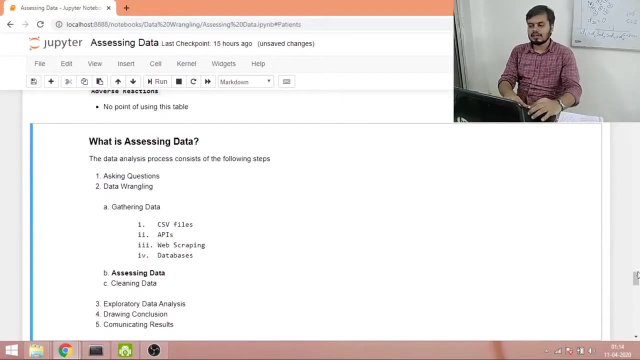 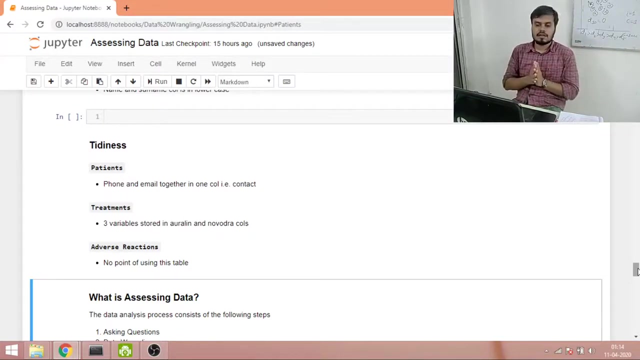 will have non-value. there is no logic to make a separate table for that. so we go down and again we write: no point of using this table, right, no need and guys, these were our three tidiness issues. we have to remove these too. ok, when we will? 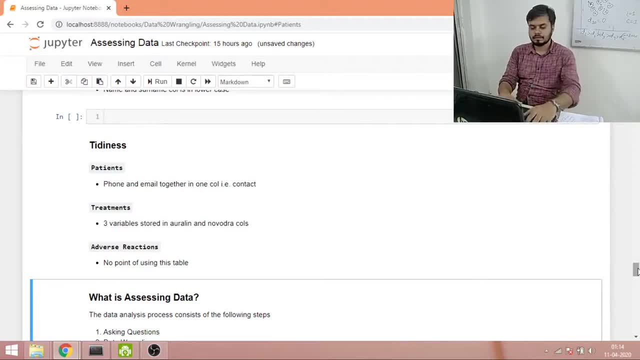 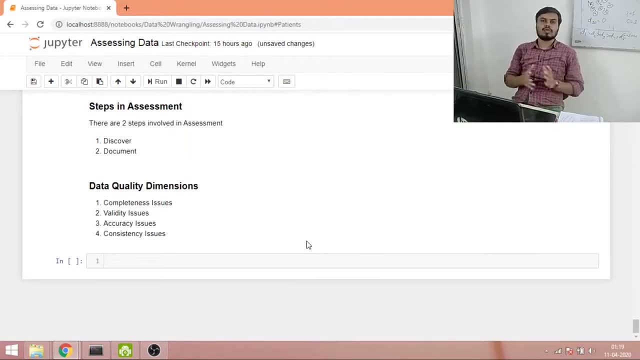 clean. so I hope everything is clear, ok, guys. so one last thing: your data quality issues. these are divided into four parts, four types of this. first is completeness issue: so data is missing, there is no data. this is completeness issue. second is validity issue: there is data, but it is not valid. 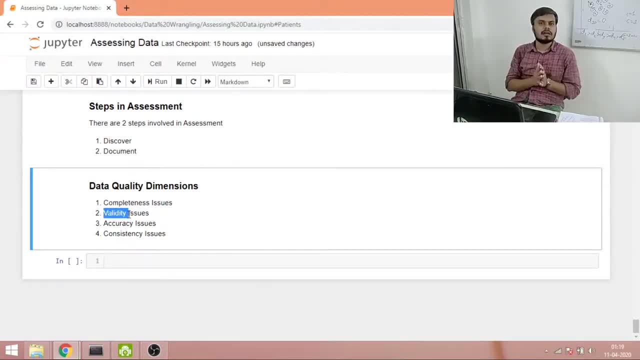 ok, it is invalid. I will give you one example: height is given in negative. this is invalid. it is not possible. third is accuracy issue. data is available as in complete. the height is one centimeter inaccurate data. there is no point of this. data ok. and the last one is: 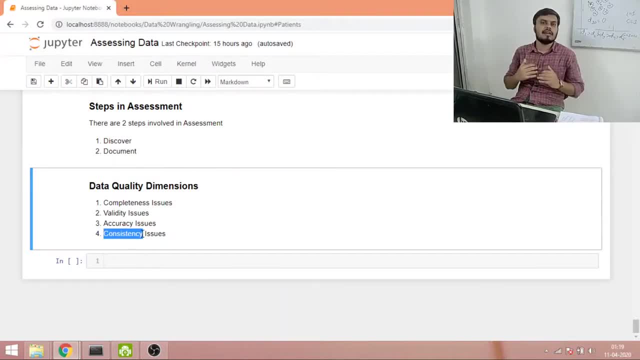 consistency issue. data is inconsistent. sometimes New York is written, sometimes NY is written. ok, so these are four dimensions. it will be beneficial to remember them that, whenever you are knowing what are the issues in your mind, you can actually- you know- call them. you can actually refer them. 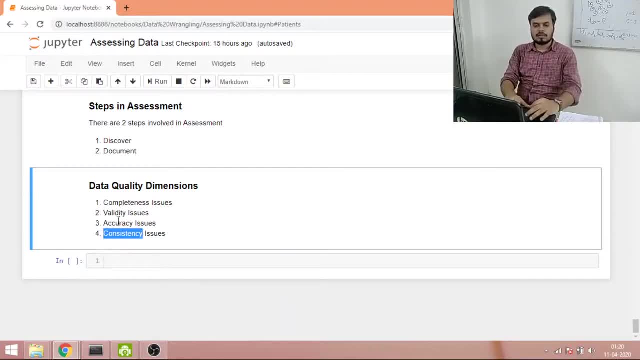 and you can see what is happening. ok, if someone asks you which one is the most serious and which one is the least serious, on experience basis, I would say completeness issue is the most serious issue. so first of all, you should think of filling incomplete data. ok, after that. 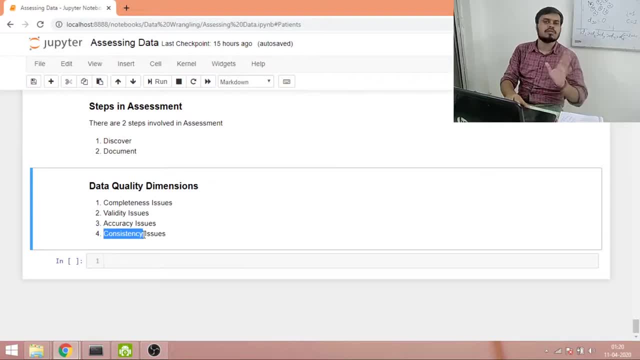 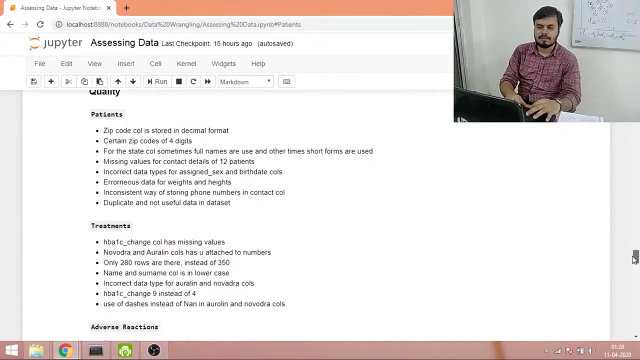 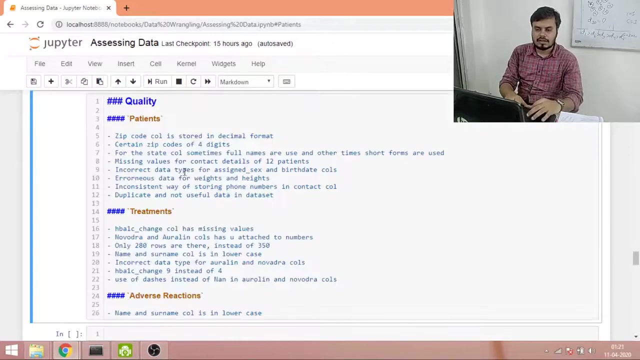 the most serious issue is validity- invalid data is bad. after that, accuracy, and then consistency. ok, all these data quality issues. I will show you all these data quality issues. we divide them in these four dimensions. it would be a good practice and good understanding will develop. so what I am? 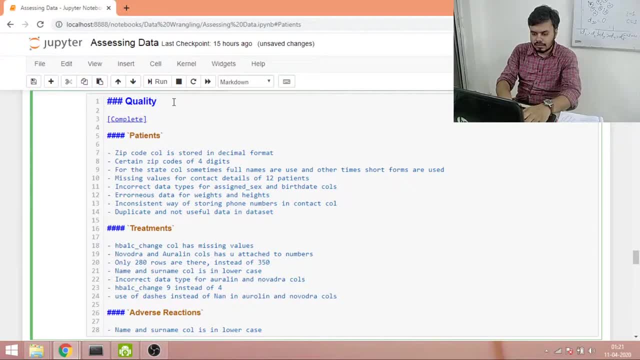 saying we will divide in these four things. so completeness, completeness, completeness, completeness. next is validity, next is accuracy and finally, consistency. ok, we are going to divide all these in these four. so the first thing is zip code. column is stored in decimal format. ok, zip code is stored in. 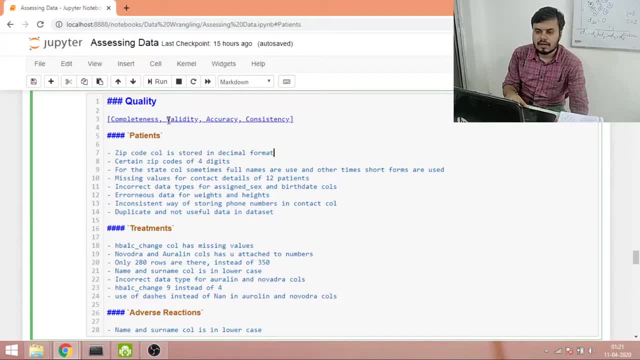 decimal completeness is not a problem, because data is complete validity. so because of that dot it will not be valid. so here either it should be validity or consistency, not consistency. this is validity. so we are putting this issue in v? v as in validity. next is certain zip codes. 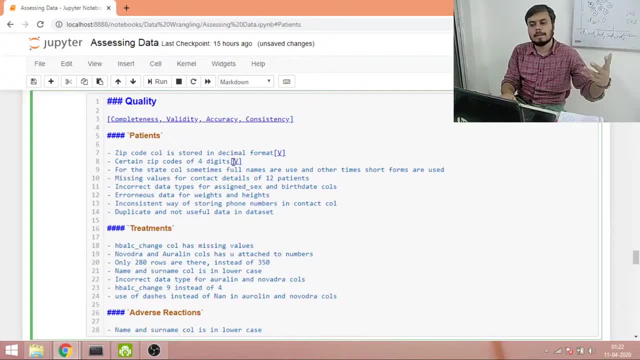 of four digits. again, it is not valid. zip code can't be in decimal, can't be in four digit zip code. sometimes full names are used, other times short forms are used. new york, ny. so we know these are consistency issues. i will write it: ic, ic as in. 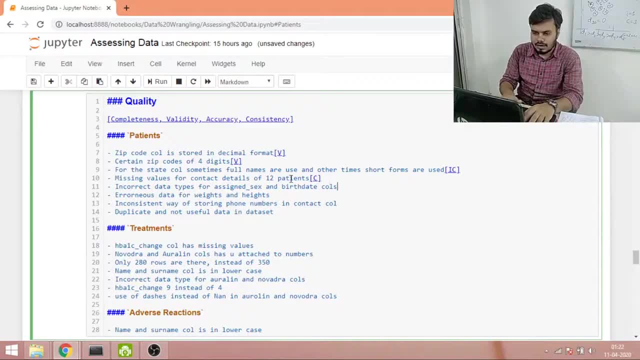 inconsistent data. next is missing values for contact details. this is very straightforward. this is completeness issue. next is incorrect data type for assigned sex. this is validity issue. data is not invalid. we have kept this. accuracy is also not going from this and consistency is also not, so this is 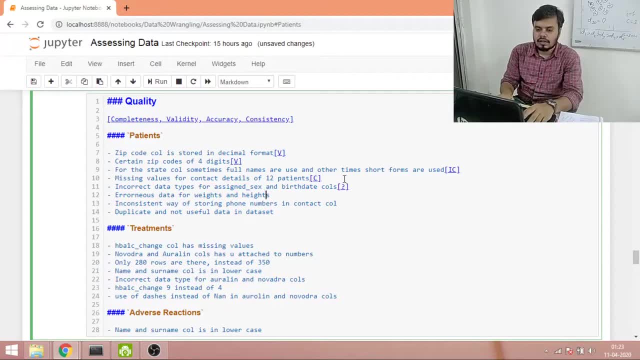 a bit of a question mark for me. you also have to think what can happen next is erroneous, ok, erroneous, this is accuracy issue. ok, because this much weight and height is not possible, so this is not accurate. inconsistent way of storing phone numbers in contact column: this is: